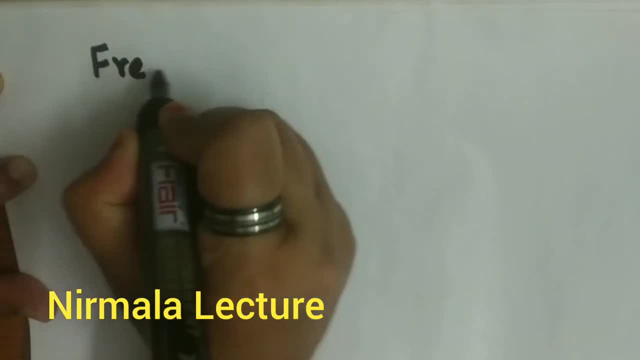 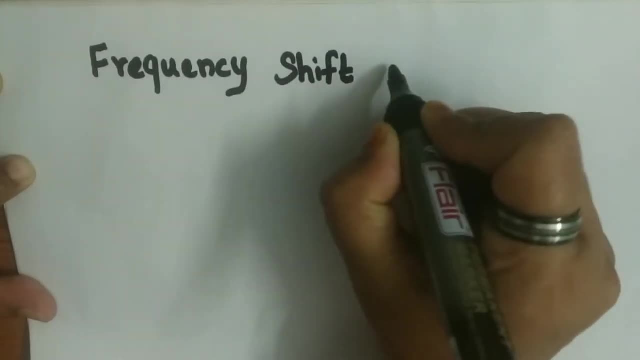 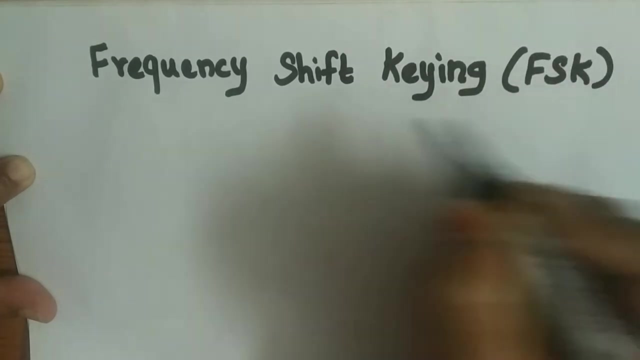 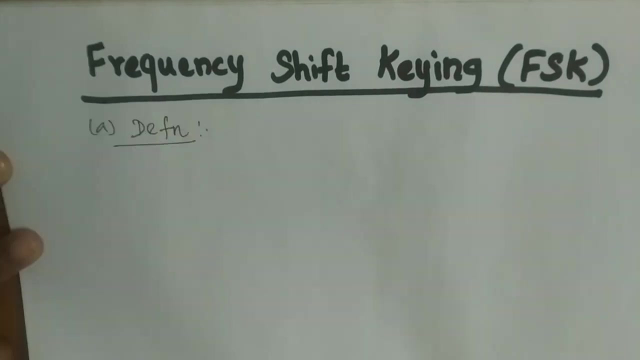 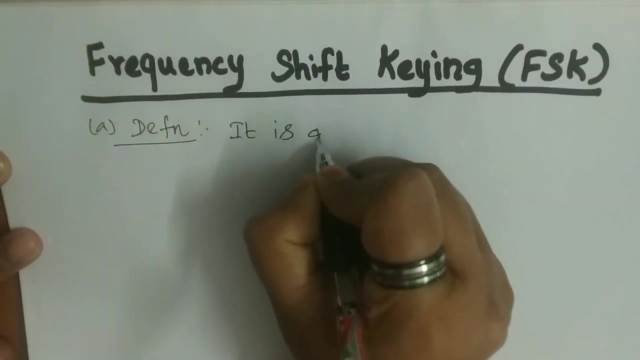 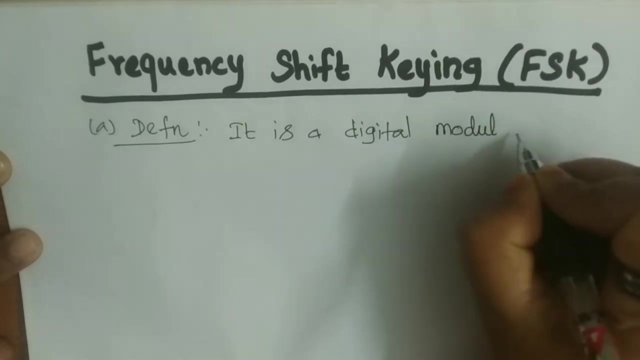 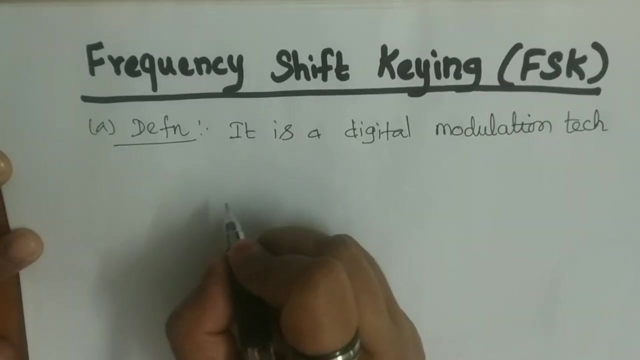 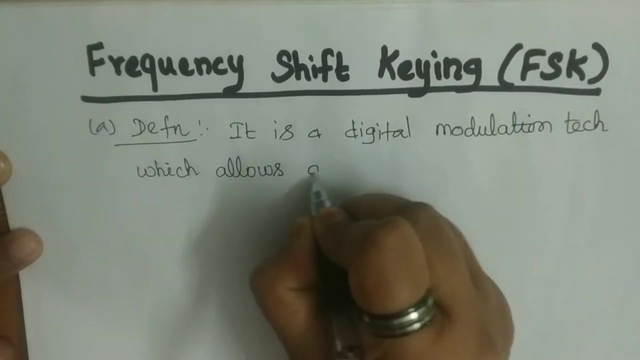 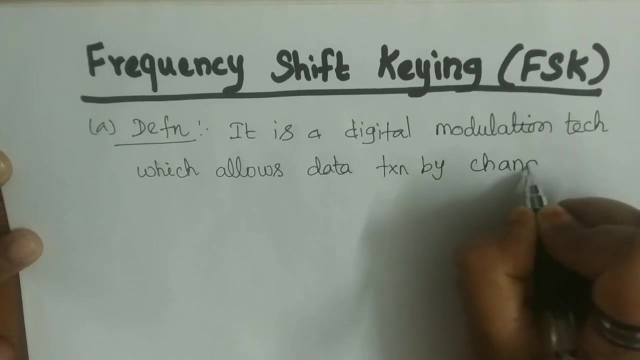 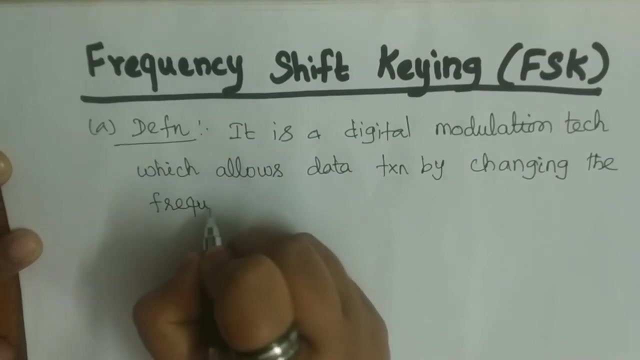 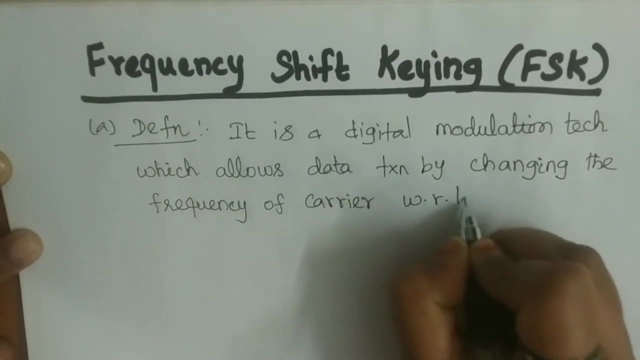 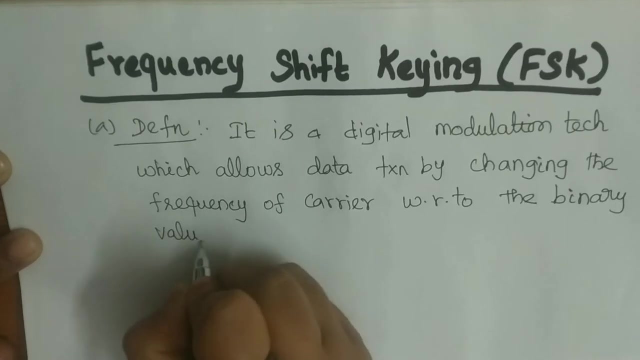 Press subscribe button below this video for more videos. Thank you. In this video we are going to discuss about frequency shift keying. It is a digital modulation technique which allows data transmission by changing the frequency of carrier with respect to the binary values of modulating signal. 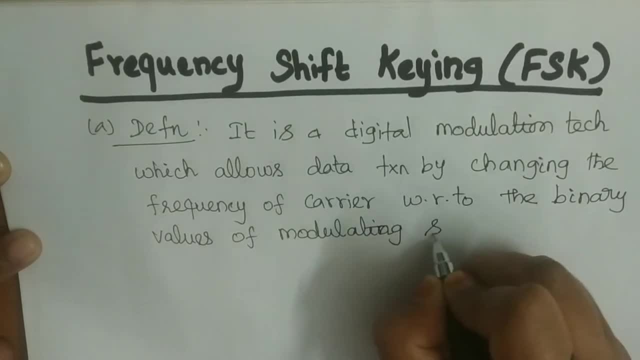 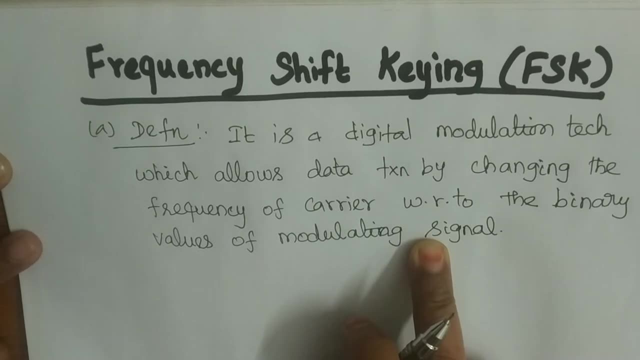 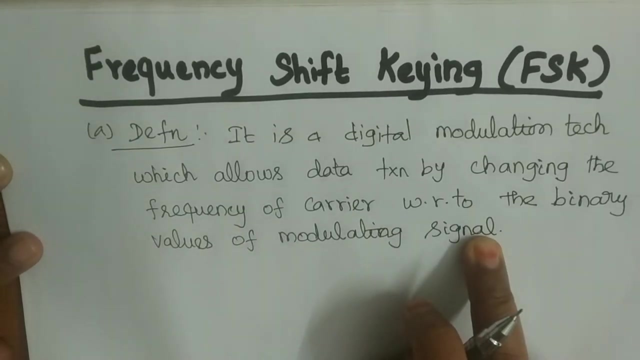 So this is the definition for frequency shift keying. It is a digital modulation technique which allows the data transmission by changing the frequency of carrier with respect to the binary values of modulating signal. Or else simply we can say that the frequency of carrier 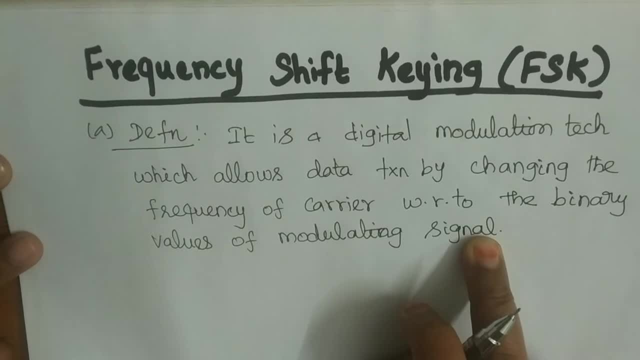 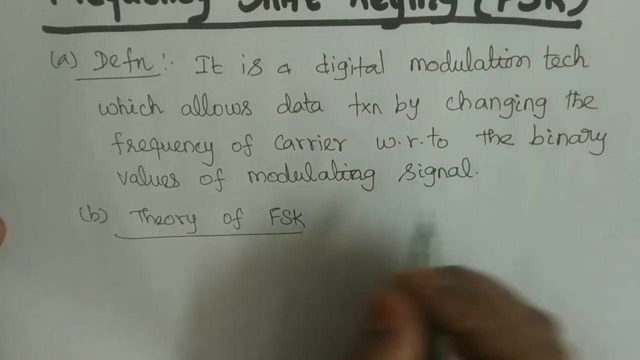 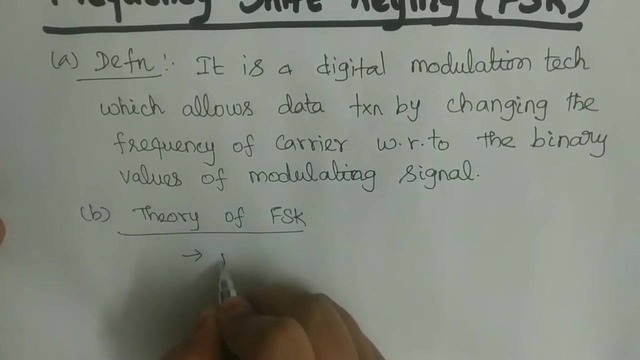 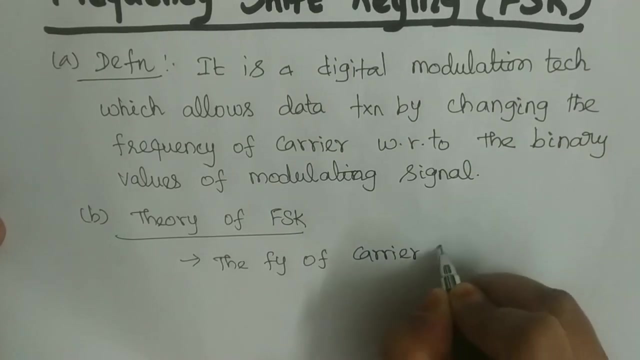 The frequency of carrier signal changes with respect to the binary values of modulating signal is known as frequency shift keying. Then we discuss about the theory of frequency shift keying. What is the definition we have to write for frequency shift keying The frequency of carrier signal. 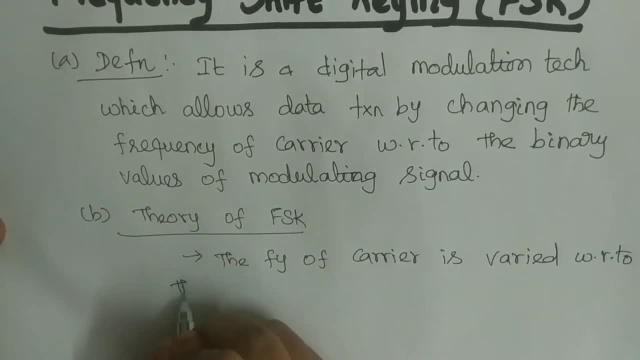 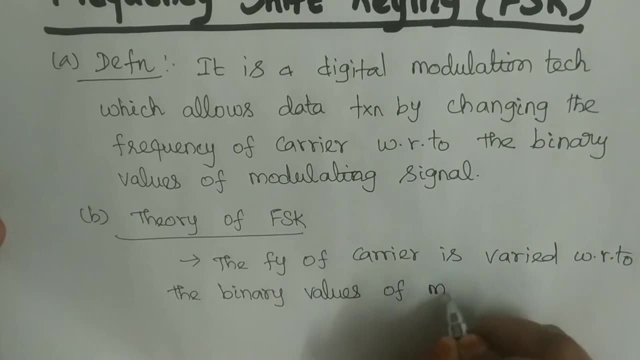 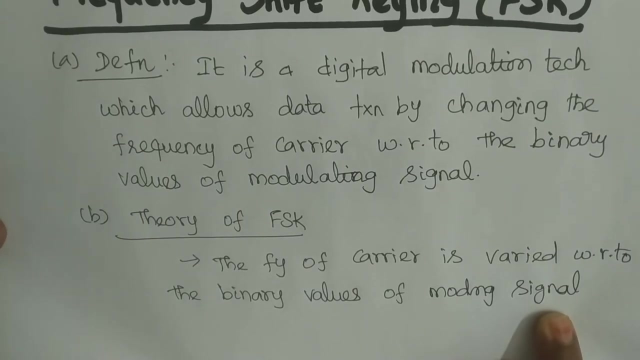 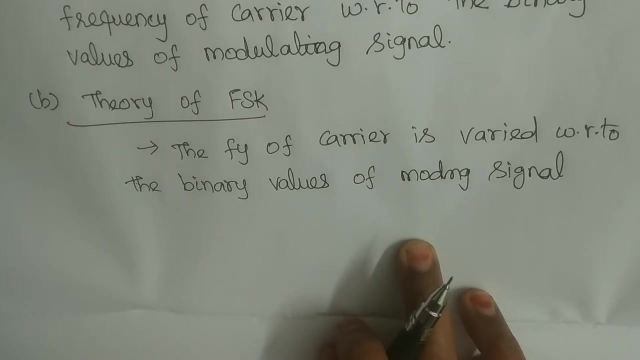 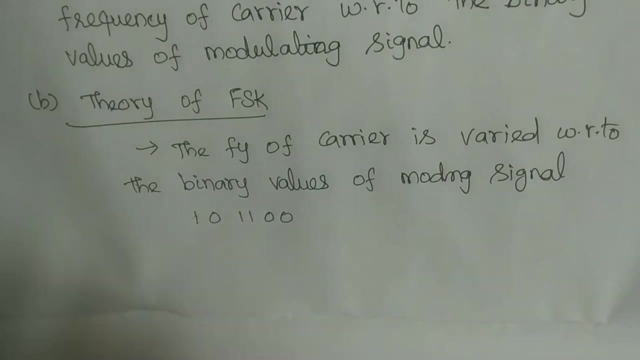 The frequency of carrier is varied with respect to the binary values of modulating signal. The frequency of carrier is varied with respect to the binary values of modulating signal is known as frequency shift keying. The frequency of carrier signal changes. So, for example, 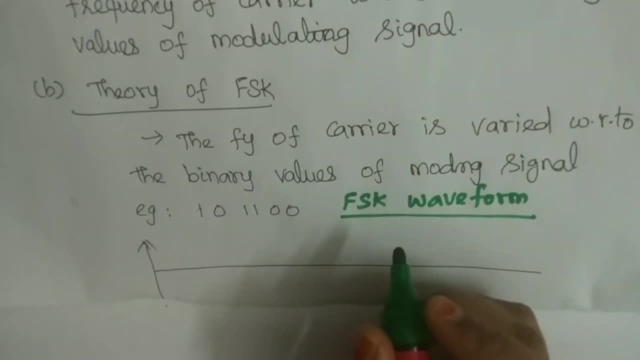 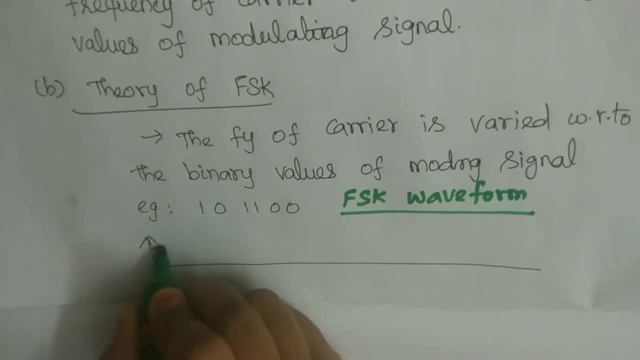 Now I am going to draw the waveform for frequency shifting. What we are going to transmit? 1, 0, double 1, 0.. 1 and this is 0, then 1, again 1, then 0, 0.. So this is what we are going to transmit. 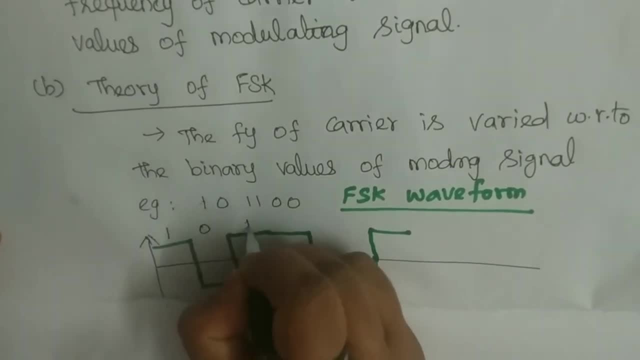 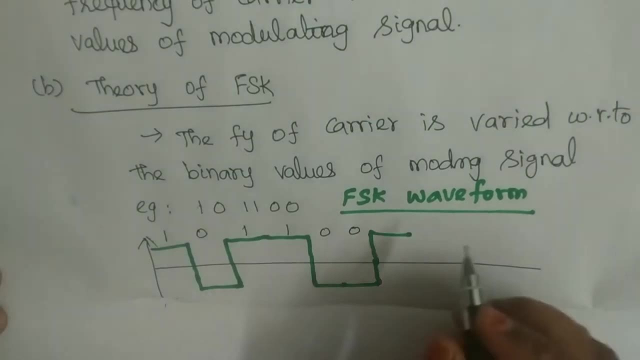 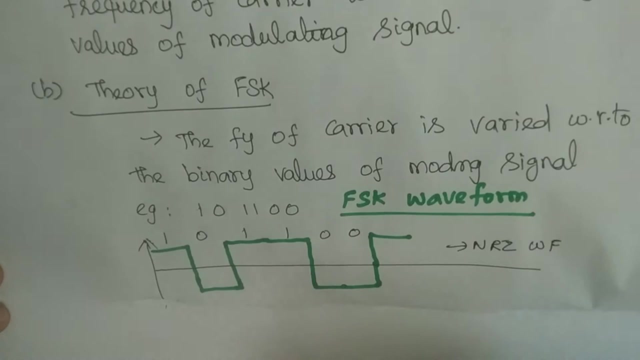 What is the data we are going to transmit? This is 1 and 0. 1 1 0, 0.. So this is n or z waveform. Here it is plus 1 and here it is minus 1 volt. This is the binary data: 1, 0 double 1 double 0.. 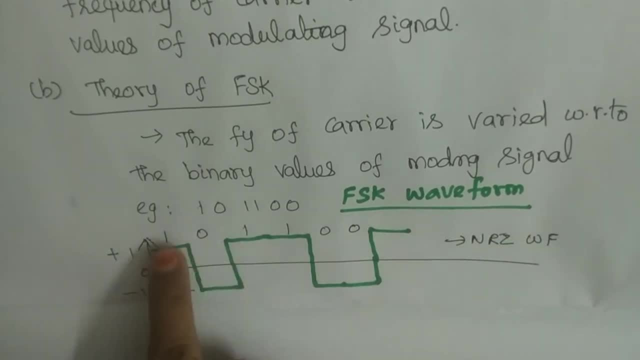 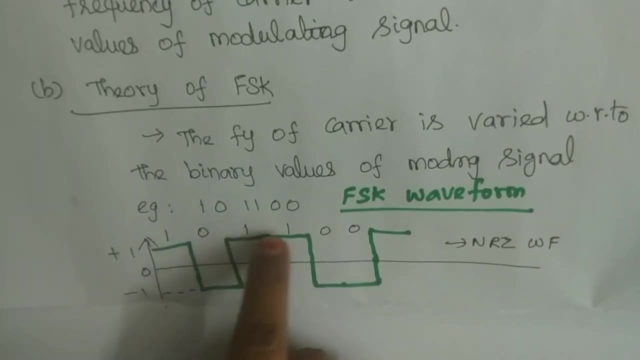 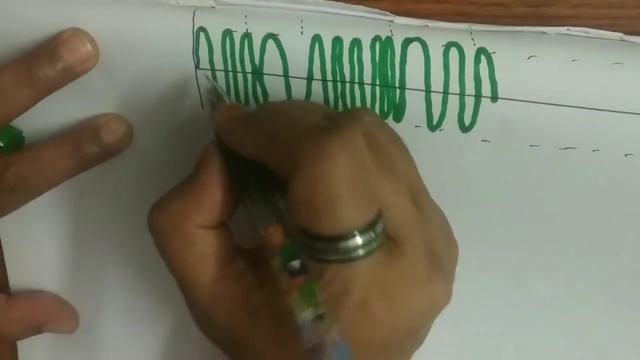 And this is the n or z waveform. This waveform is on waveform corresponding to binary data: 1.. This is 0 of waveform. This is 1. again 1, 0, 0.. And this is frequency shifting waveform. For 1, we are getting the waveform like this: 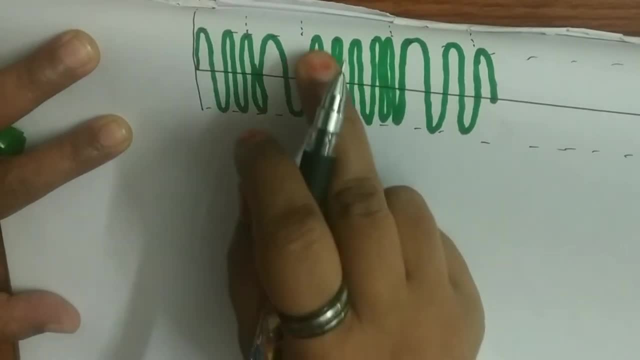 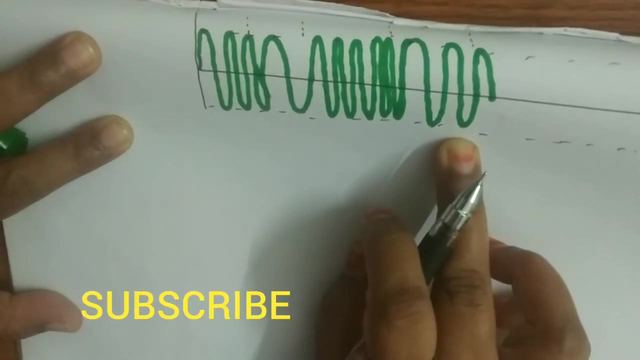 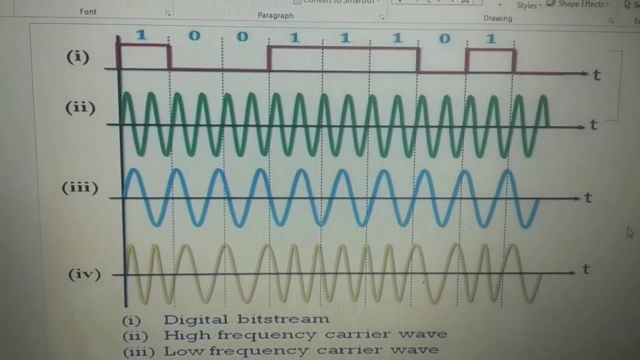 For 0, we are getting the waveform, Then again 1, then again 1. For 0. The frequency is increased. So in this way we have data: 1, double 0, triple 1, 0, 1.. So this is example waveform. 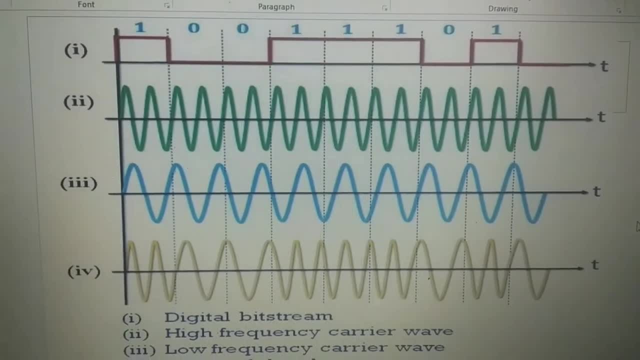 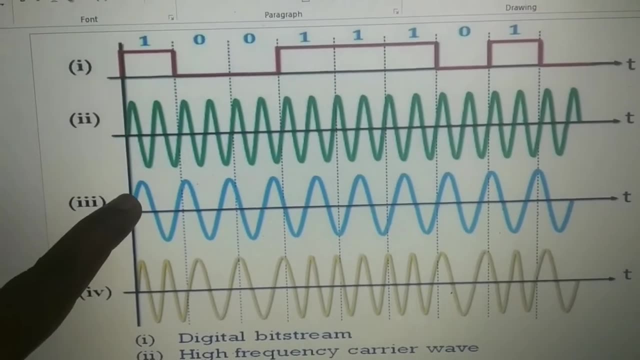 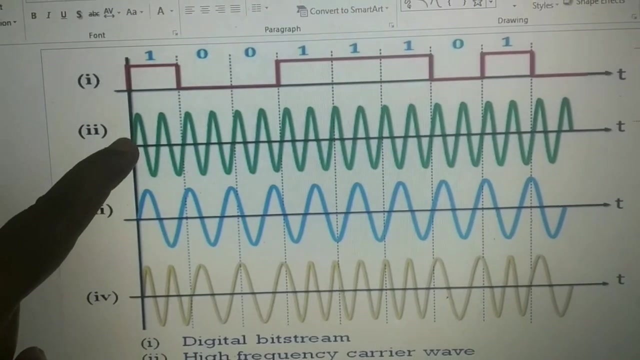 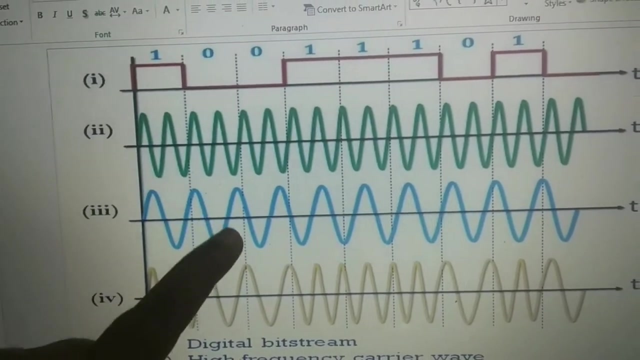 The first waveform represents the n or z waveform, And here this is the normal carrier signal, And this is high frequency carrier signal. This is high frequency carrier signal. This is low frequency carrier signal. This is low frequency carrier signal. If we are transmitting 0, we have to draw the waveform like this: 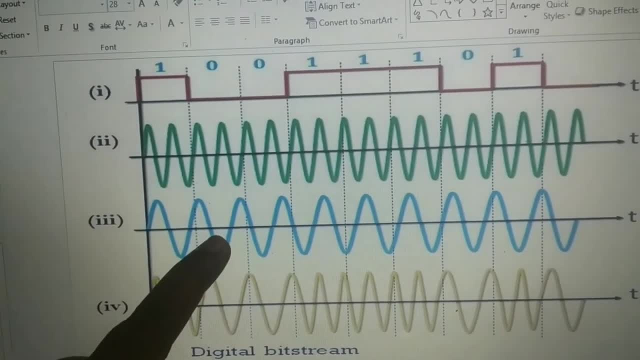 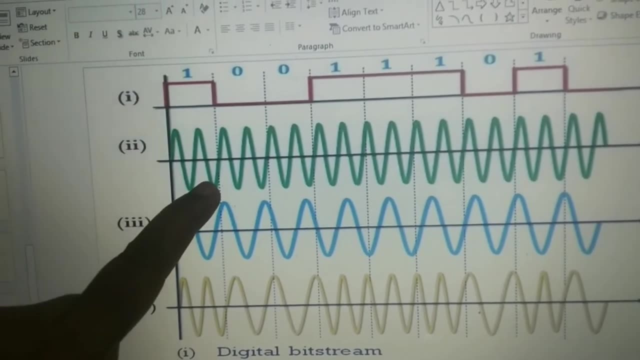 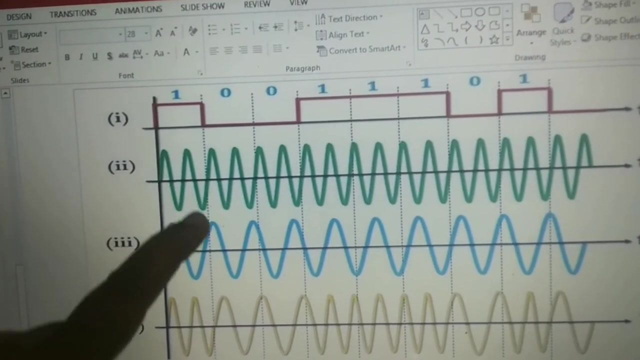 See for 0, number of cycles may be decreased, Isn't it? For 1, number of cycle is increased. For 1 cycle, the number of cycle is 2 cycles. Almost 2 cycles are there. For 1, the number of cycle is increased. 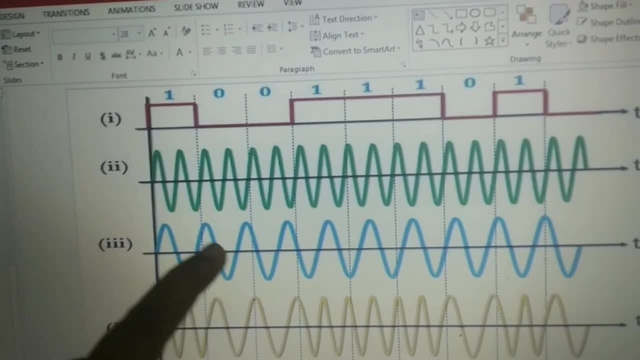 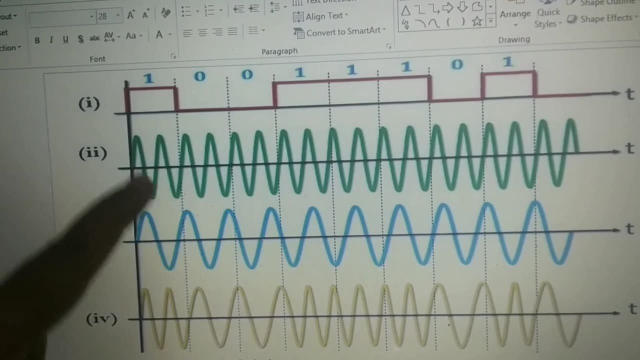 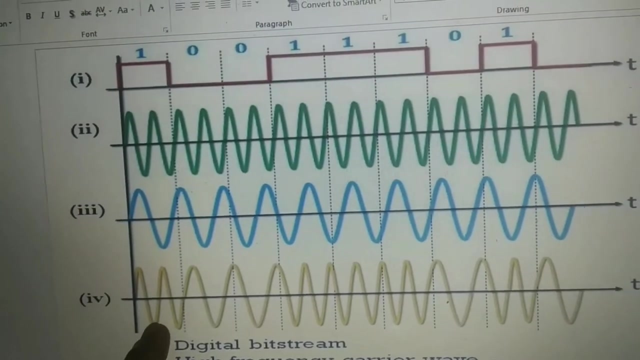 Almost 2 cycles are there. For 0,, the number of cycle is almost 1.. Isn't it So? For high frequency, the number of cycle is increased. For low frequency carrier, the number of cycle is decreased. So this is the FSK waveform. 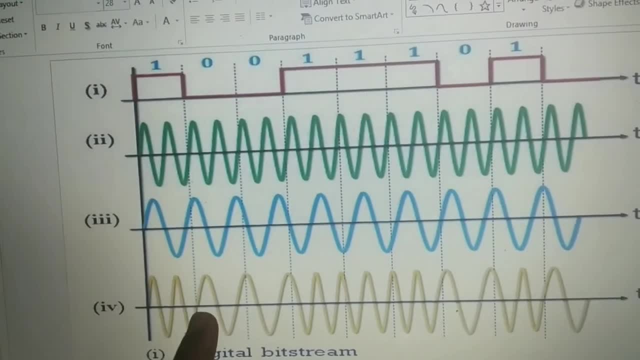 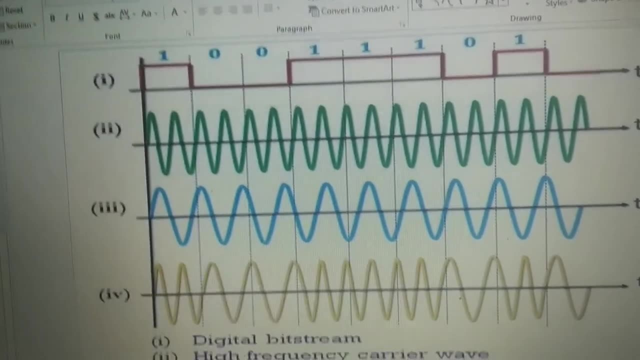 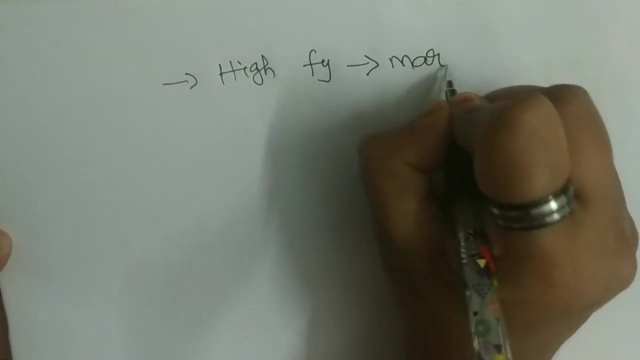 For 1,. almost we have to draw 2 cycles For 0, 1 cycles are there, So in this way we have to draw the FSK waveform L a, smorg frequency And low frequency. A is referred as space frequency. 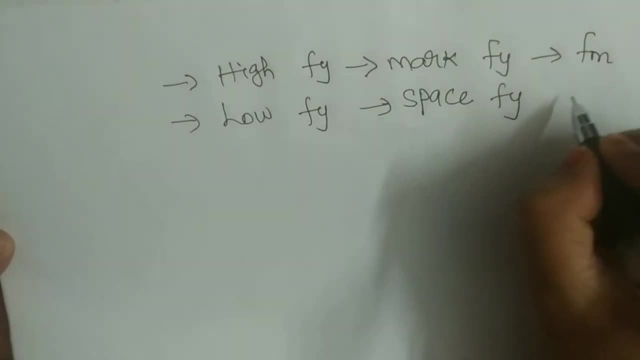 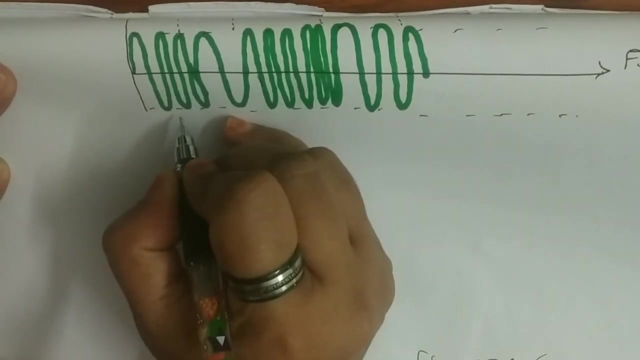 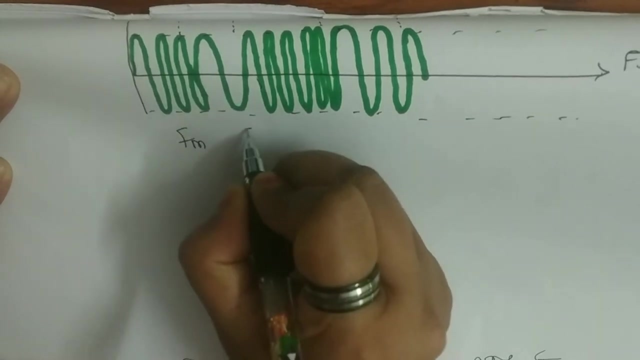 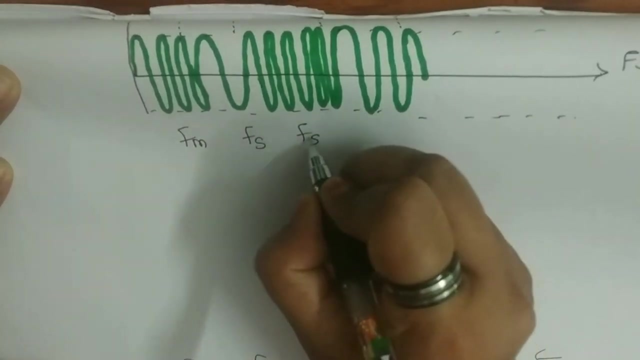 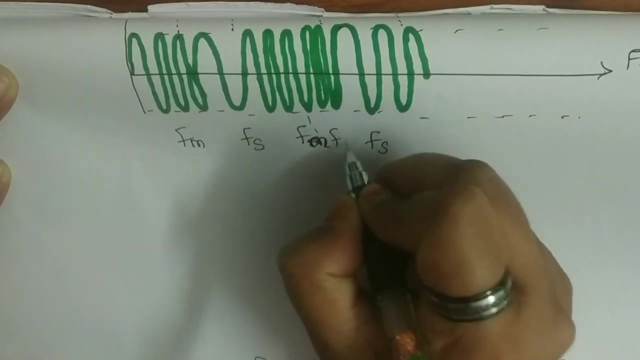 Morg frequency is represented by FM, Space frequency is represented by FS. So this is high frequency FM And this is low frequency Space frequency FS. this is high frequency FM and this is low frequency FS. And this is also. we have 2 high frequencies. 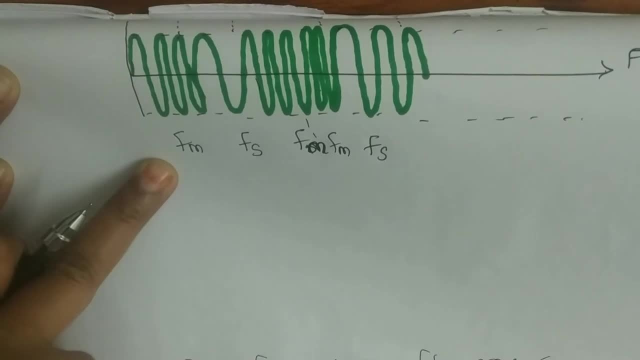 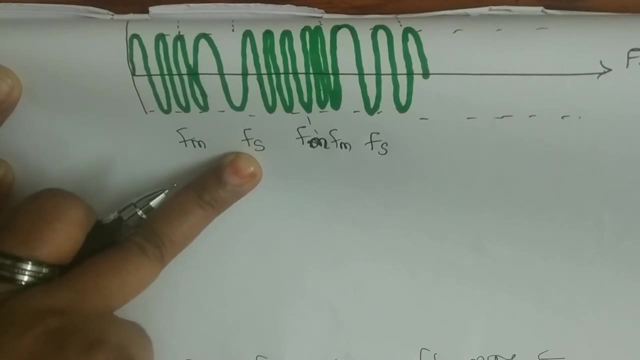 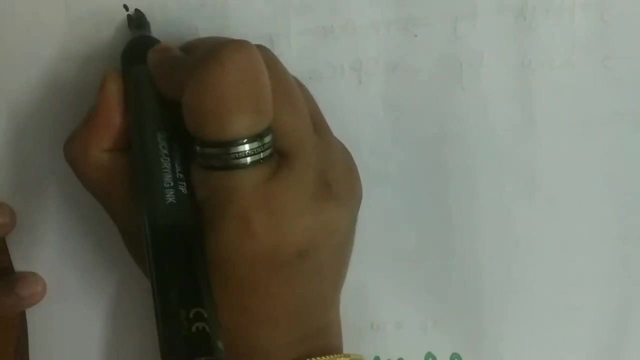 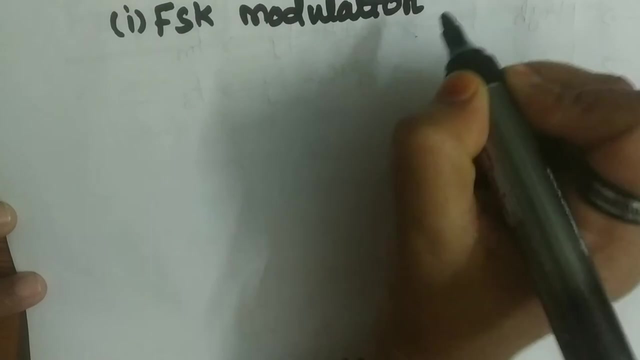 And FM represents the high frequency, which is referred as smorg frequency FS represents the low frequency, which is referred as space frequency FS, And low frequency FM represents the low frequency FSK modulation. It's nothing but FSK transmitter. 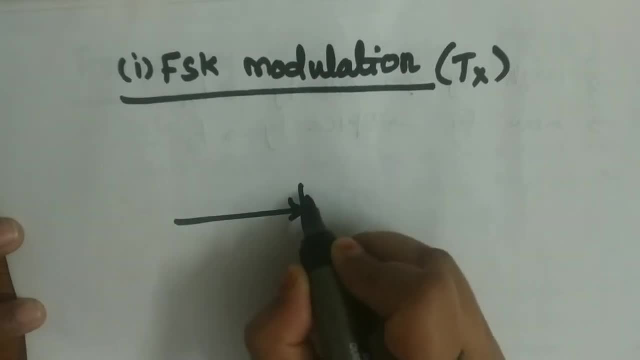 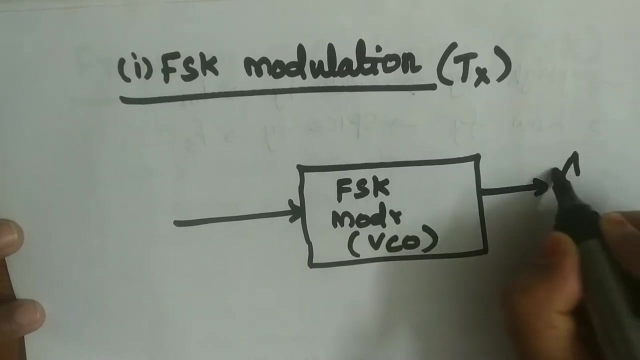 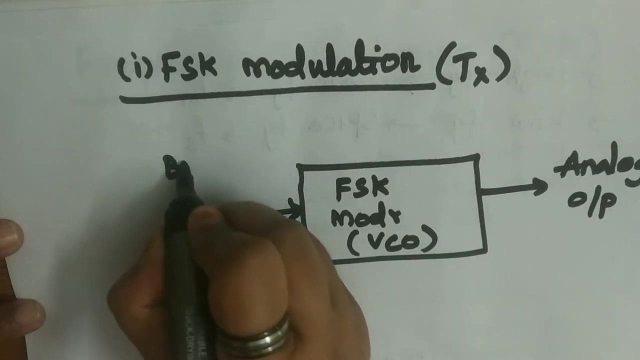 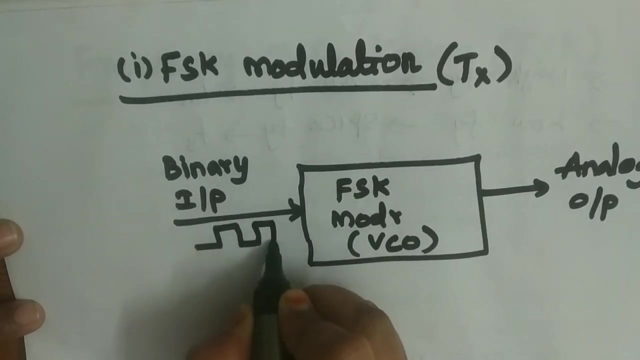 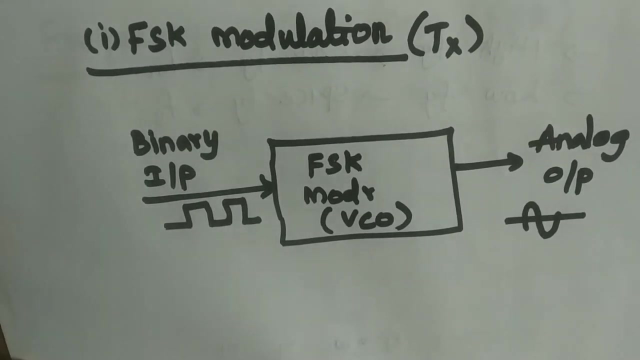 So this is how it looks. So this is the simple block diagram of FSK modulator or FSK transmitter. 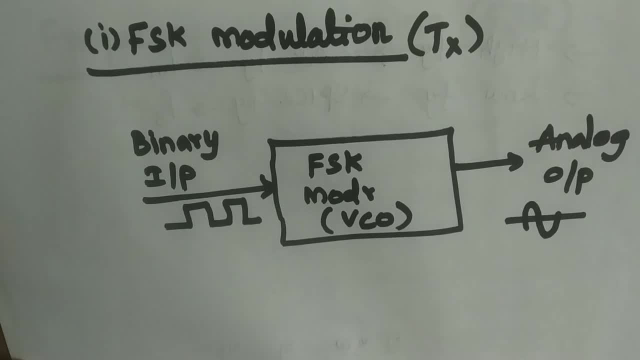 So here voltage controlled oscillator is used as a FSK modulator. Voltage controlled oscillator is used as a FSK modulator. Here we are giving the binary input From VCO. we are getting analog output. So FSK waveform is the output for voltage controlled oscillator. 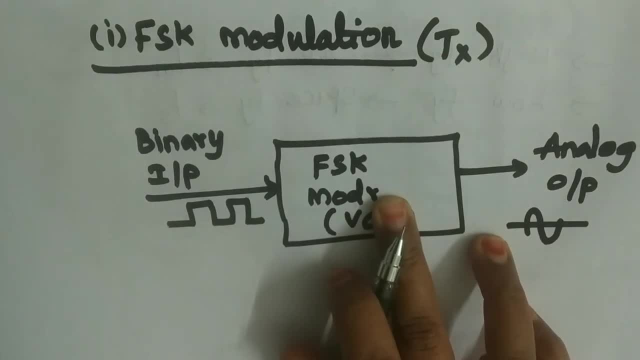 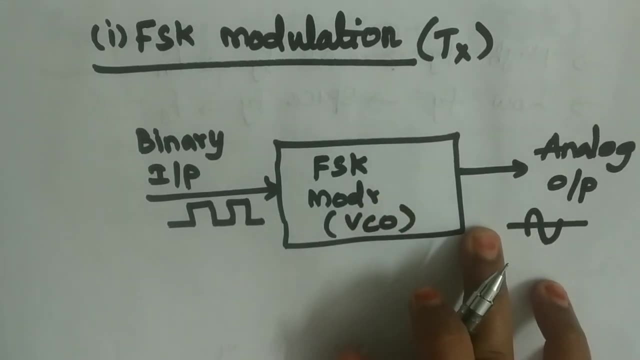 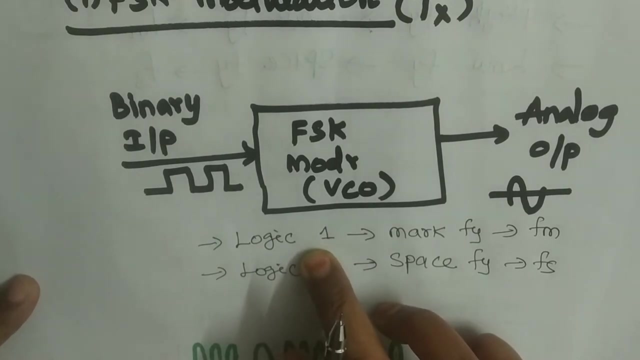 It will generate a different frequency based on the binary input. Then the FSK modulator output is analog output. Here, logic 1 is high frequency, which is referred as mark frequency, which is represented by FM. Logic 0 is low frequency, referred as phase frequency, represented by FS. 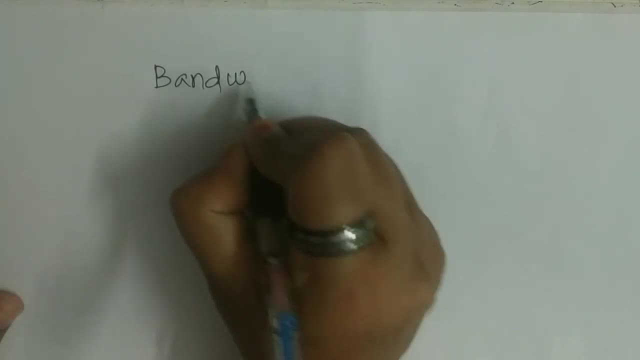 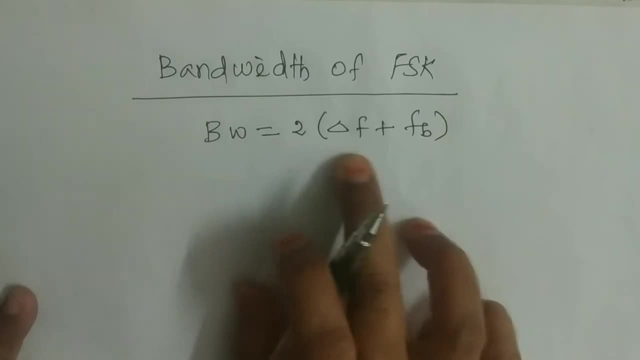 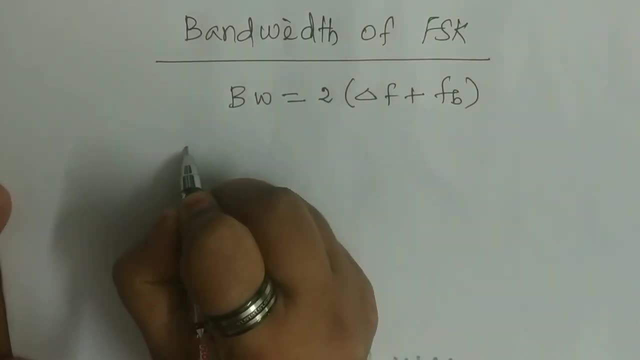 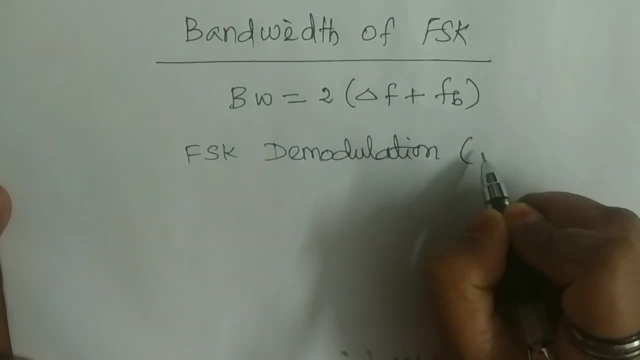 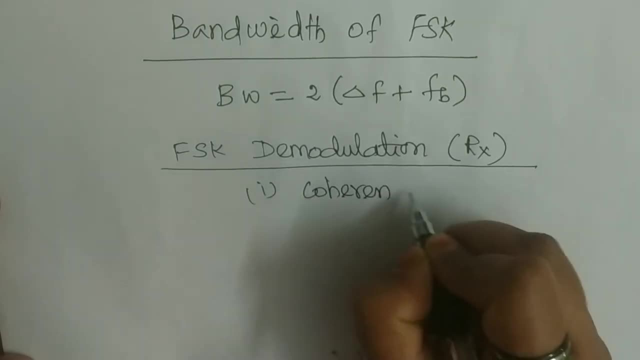 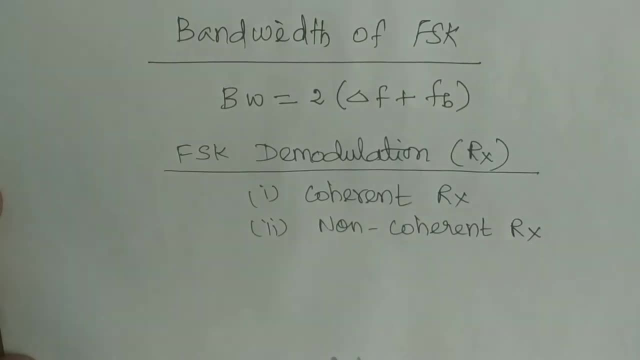 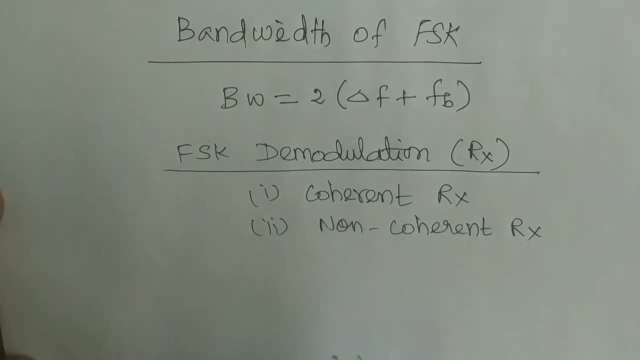 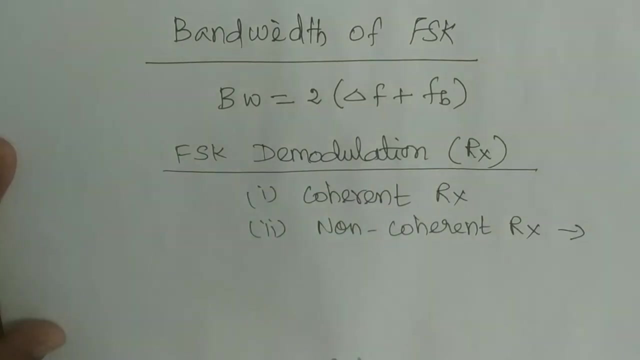 Coherent receiver and non-coherent receiver. So here we have multi-level FSK For non-coherent receiver, no carrier signal is needed. No carrier is needed for non-coherent receiver. For coherent receiver we need a carrier signal. 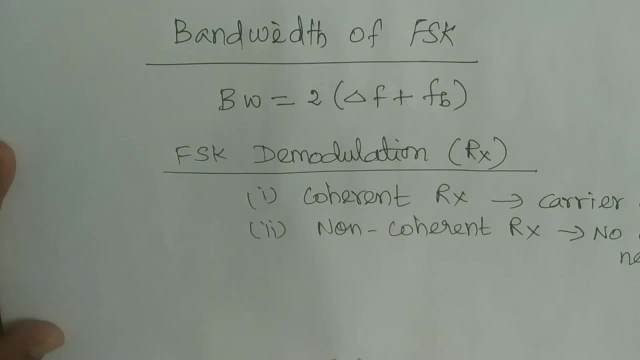 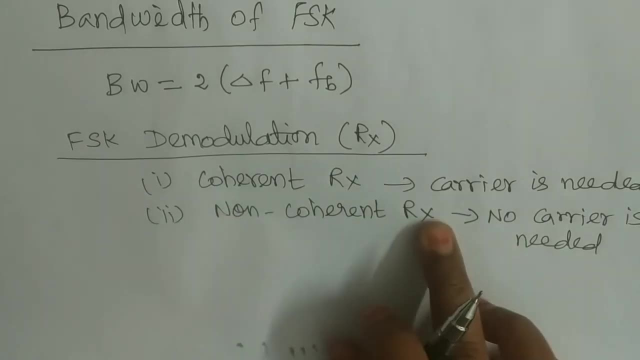 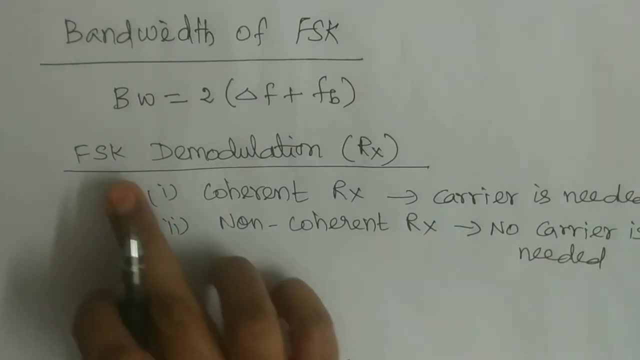 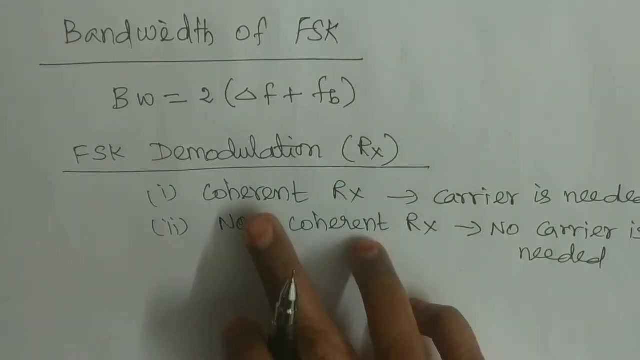 So carrier signal is needed for coherent receiver circuit. Non-coherent receiver we do not require, we don't know. For FSK demodulation technique we have two different types of receiver circuit. One is non-coherent receiver and the other one is coherent receiver. 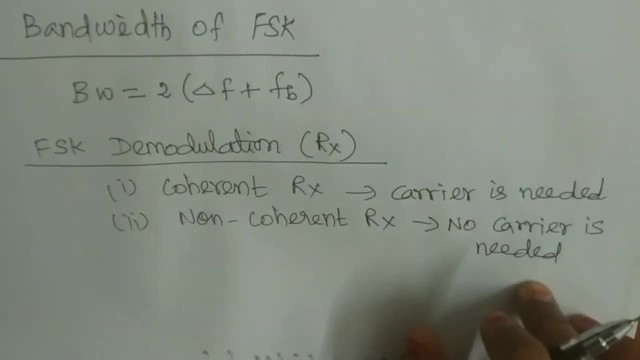 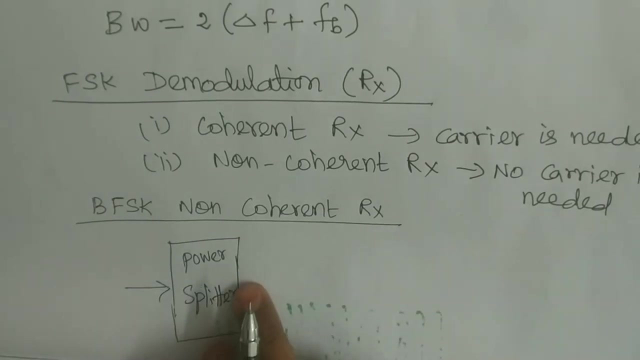 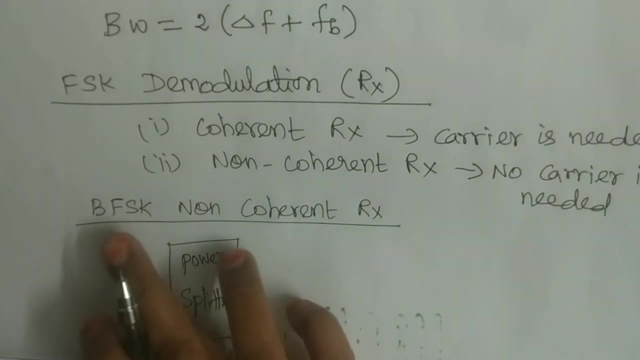 For non-coherent receiver, no carrier is needed. For coherent receiver, carrier signal is needed. Okay, So this is the block diagram of non-coherent receiver. FSK is also called as BFSK, because the carrier signal is changes with respect to the binary values of modulating signal. 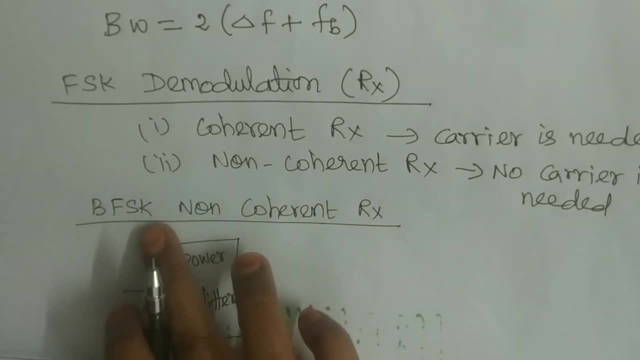 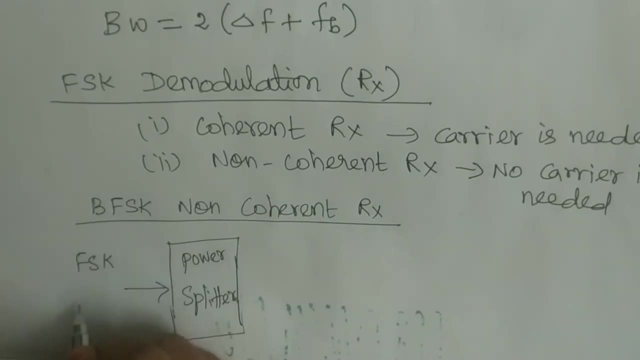 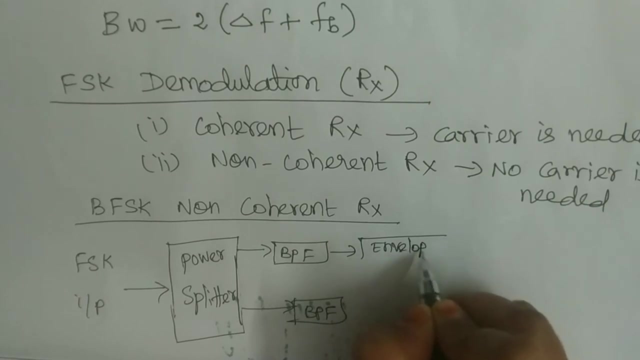 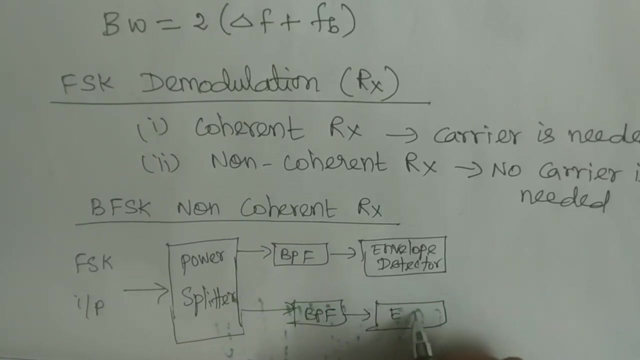 So it is also called as binary frequency shift decaying. So this is the non-coherent receiver diagram We are taking here FSK input and band pass filter- Here also one band pass filter, Then envelope detector- Here also envelope detector. 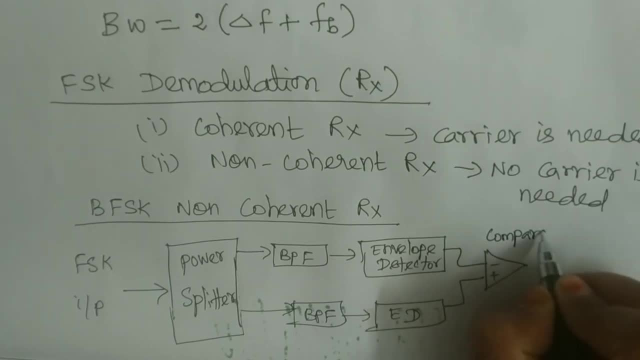 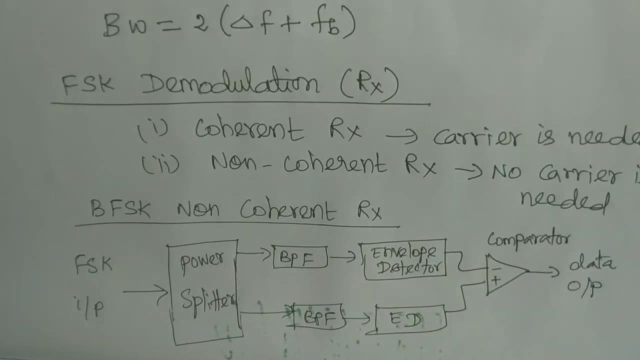 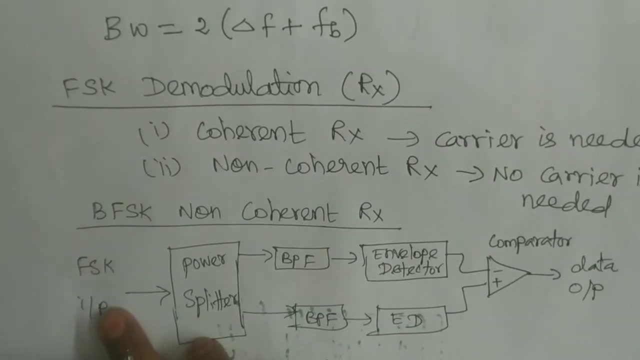 This is comparator. This is comparator. This is comparator Here: data output. So this is the non-coherent receiver block diagram. Here the input is binary shift decaying. Sorry, FSK input. Input data is FSK waveform. We are applying FSK waveform to the power splitter. 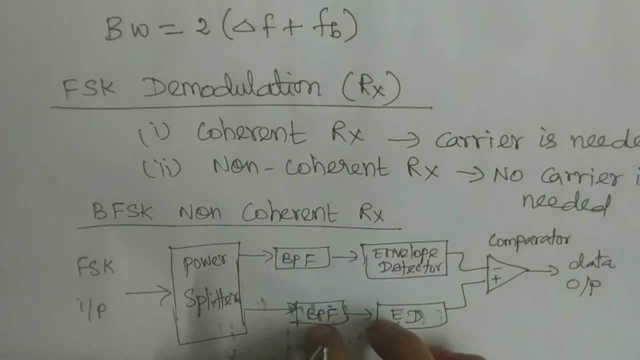 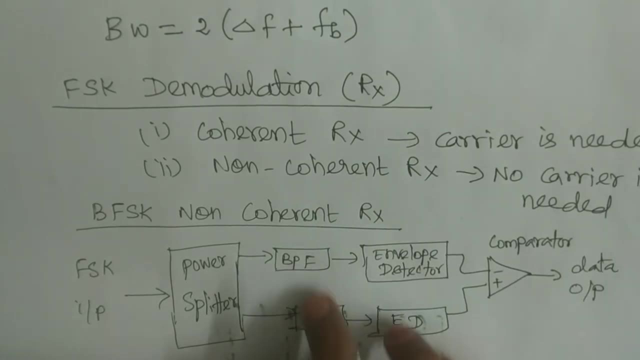 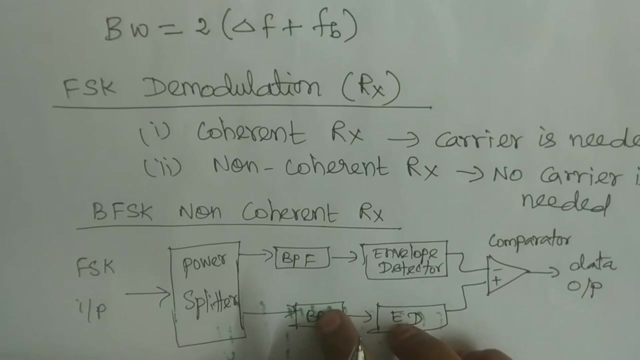 Then it is passes to the band pass filter. The band pass filter can pass only the more frequency or space frequency to its envelope detector. Okay, So the signal coming from the upper band pass filter and the lower band pass filter is applied to the upper envelope detector and the lower envelope detector. 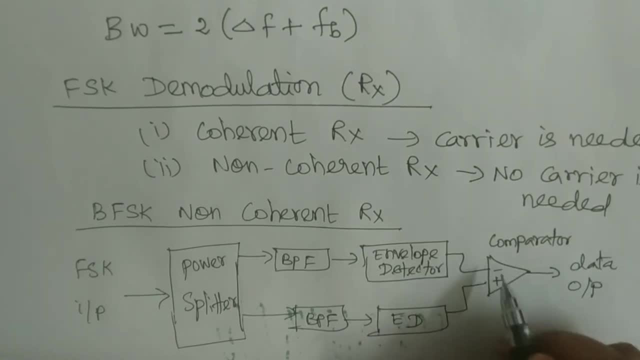 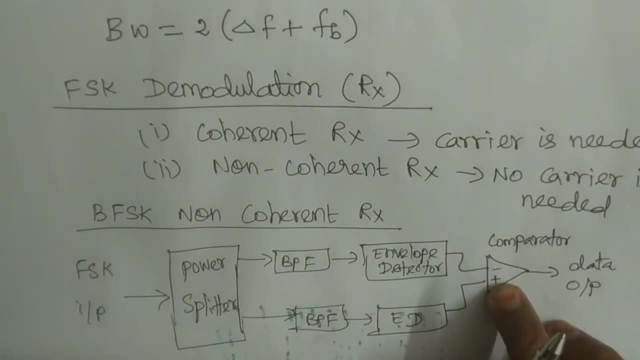 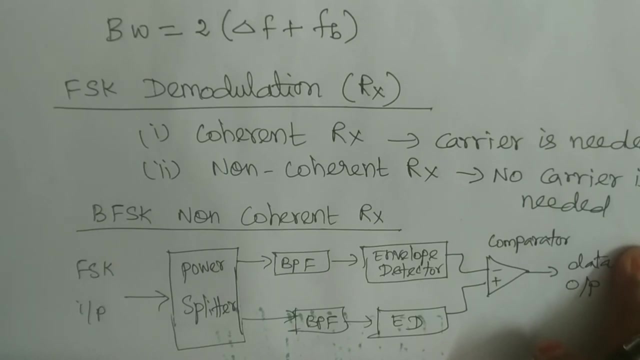 Then it is. output of envelope detector is applied. Now let's apply the same thing to the comparator. The comparator will compare the data. So in this comparator we are setting one threshold value. If it is greater than 0, it is referred as more frequency. 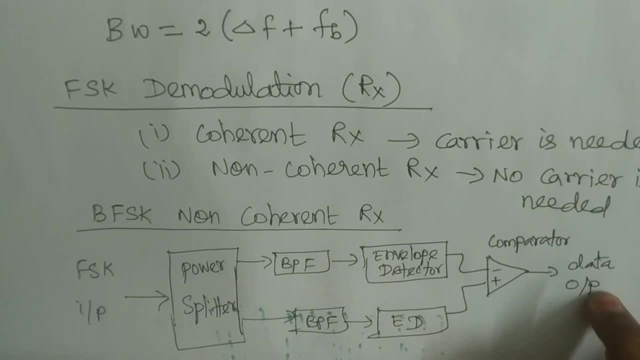 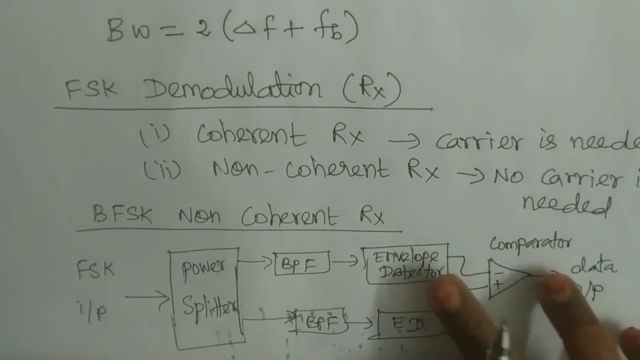 If it is less than 0, it is referred as space frequency. It means that if it is greater than 0, it is high frequency, If it is less than 0, low frequency signal can be obtained. Or else simply we can say that if the incoming data of comparator is greater than 0,, then it is considered as logic 1.. 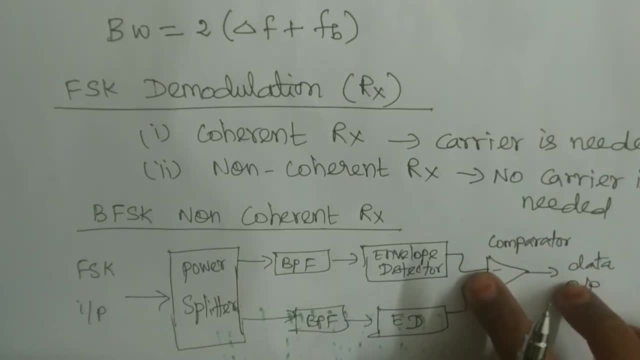 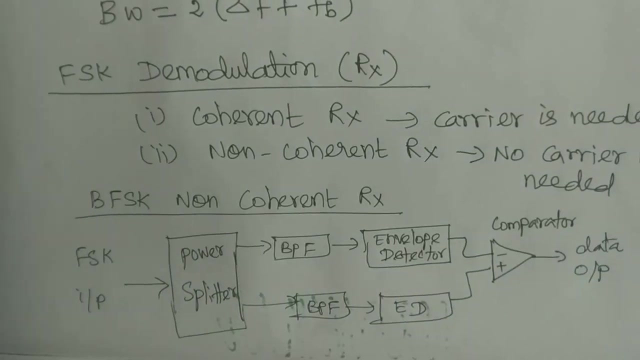 The incoming data of comparator is less than 0, then it is considered as logic 0. So in this way we are getting the corresponding binary data at the output of non-coherent receiver. See once again I am explaining the operation of non-coherent receiver. 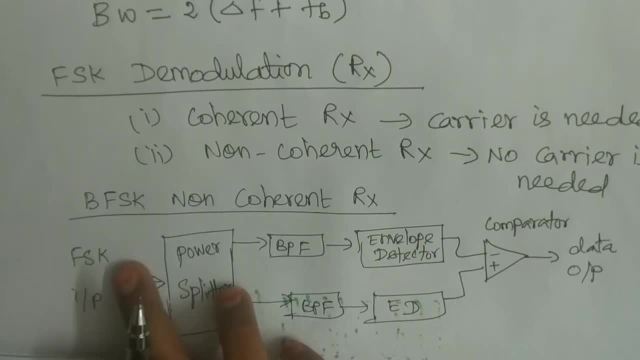 Here we are applying the FSK waveform at the input of power splitter. Power splitter split the signal. One signal applied to the upper bandpass filter and the another signal is applied to the lower bandpass filter. The bandpass filter passes the corresponding output to the corresponding envelope detectors. 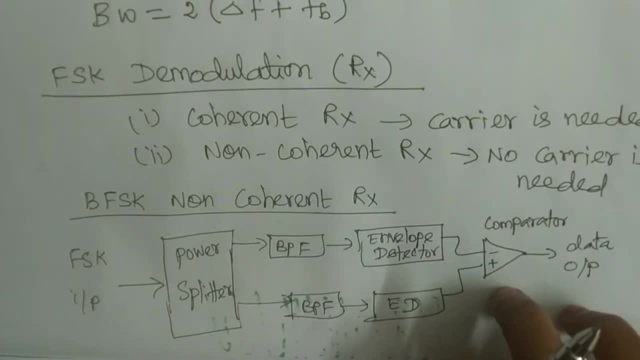 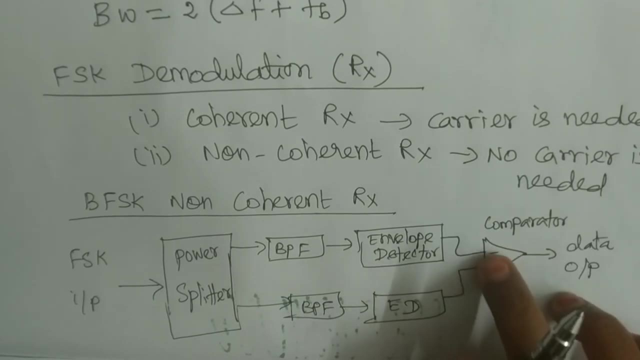 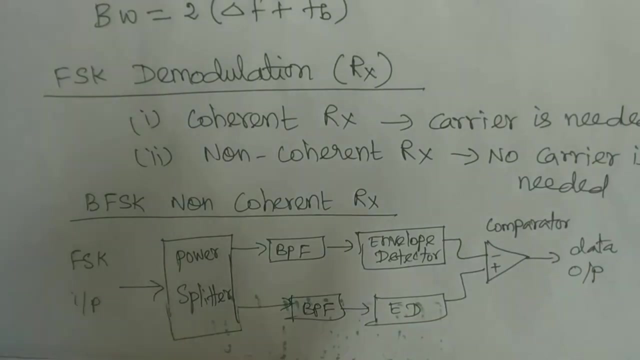 The output from the envelope detector is applied to the comparator signal. So in this comparator we are setting one threshold value. If the incoming value of the comparator is greater than 0,, then it is considered as logic 1.. If it is less than 0, then it is compared as logic 1.. 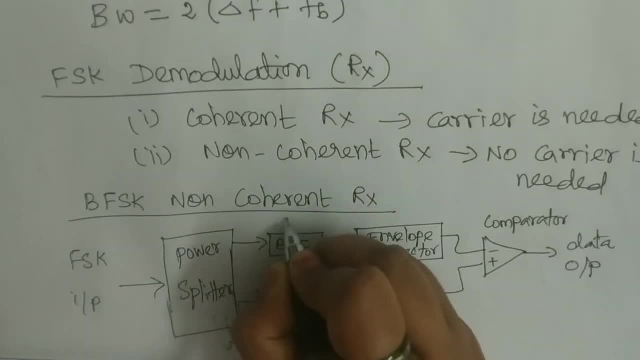 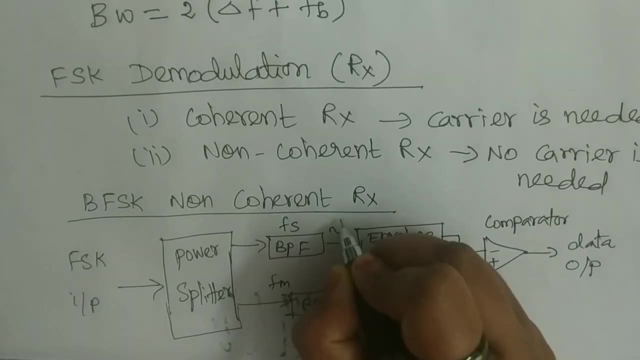 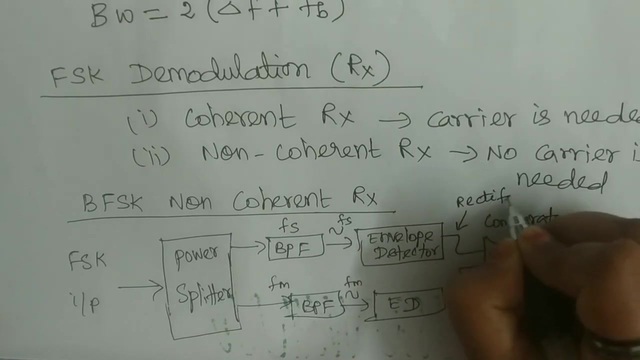 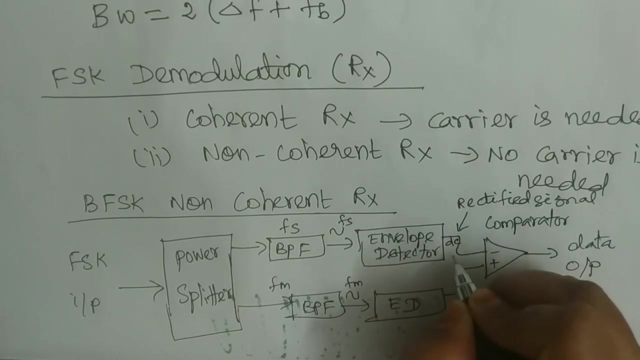 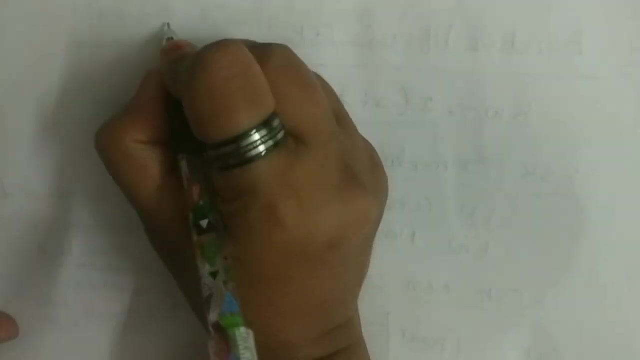 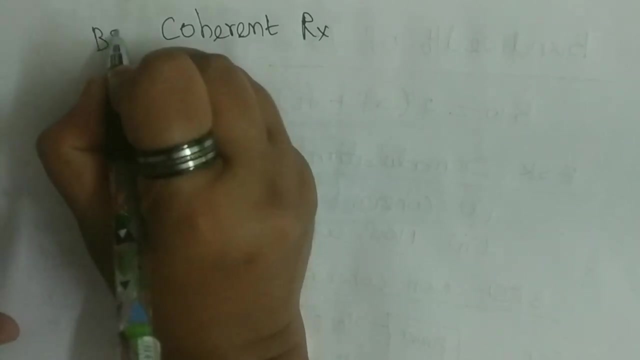 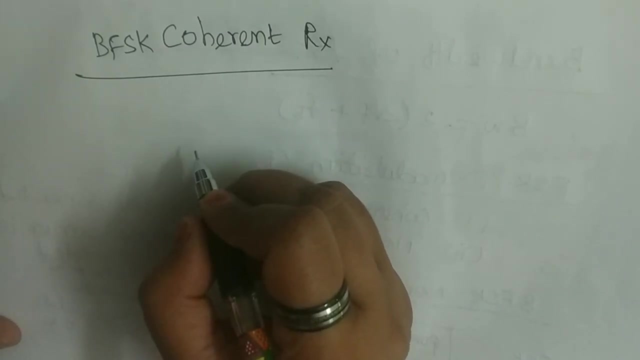 This is FM and this is FS. space frequency: This is FS and this is FM. FM: This is FS. Then here we are getting the rectified signal DC level. Then I am going to draw the block diagram of a coherent receiver: binary FSK. coherent receiver. 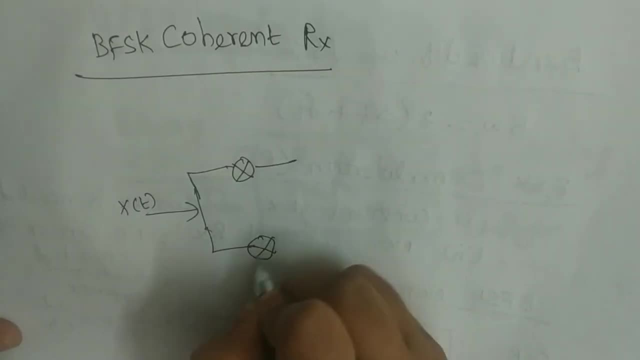 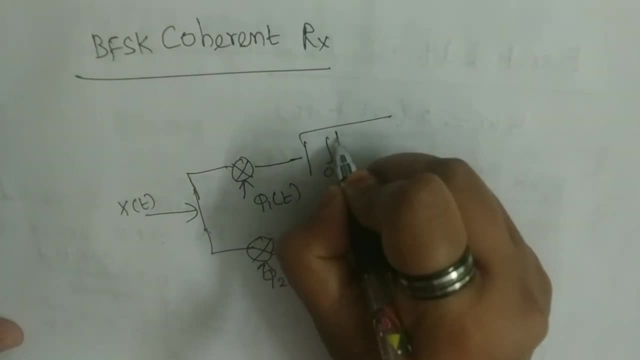 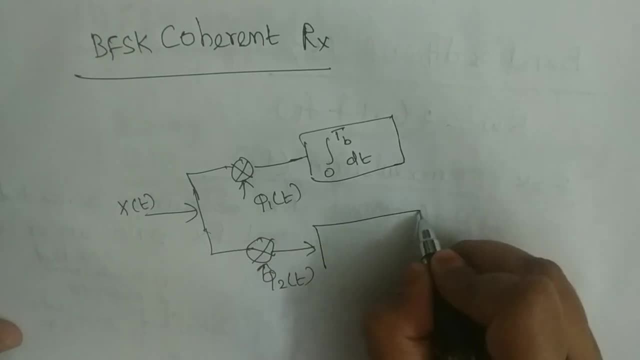 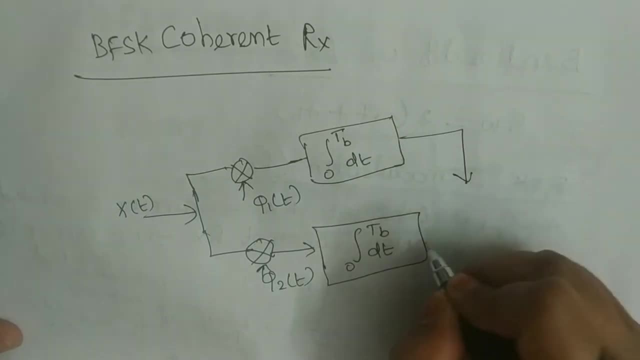 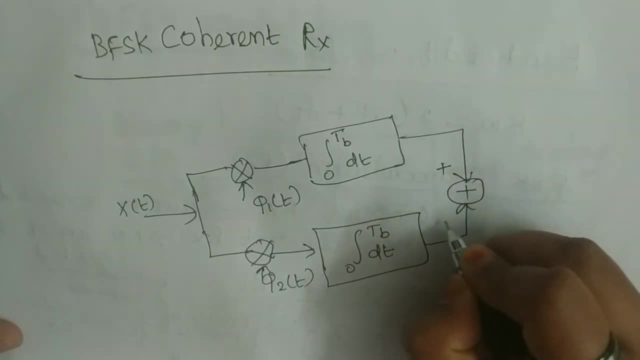 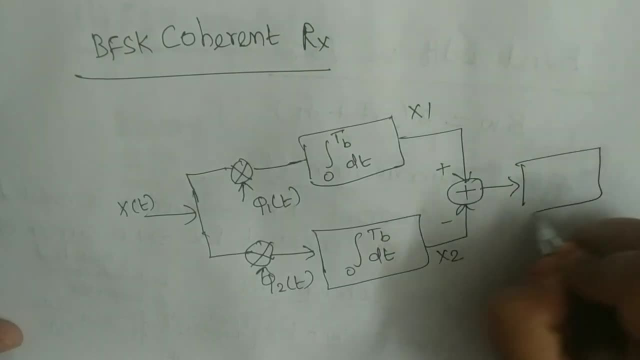 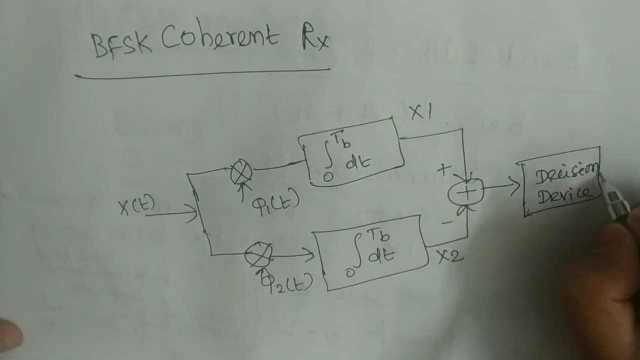 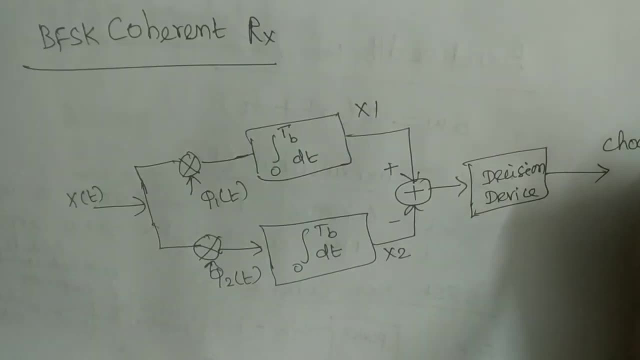 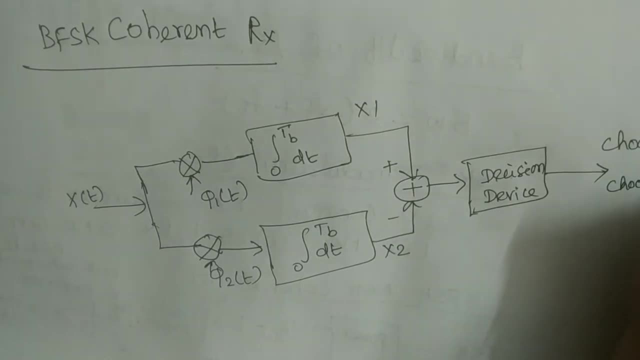 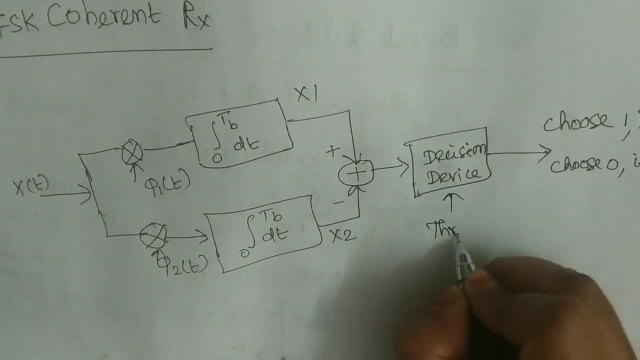 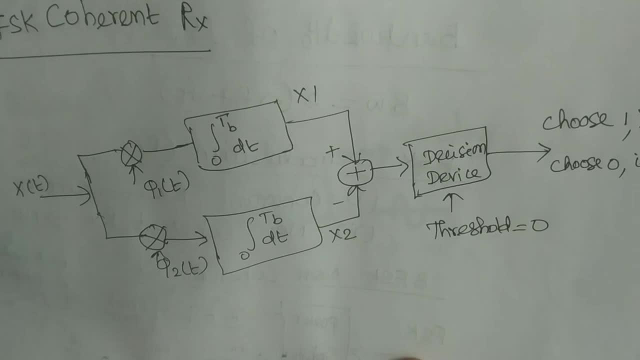 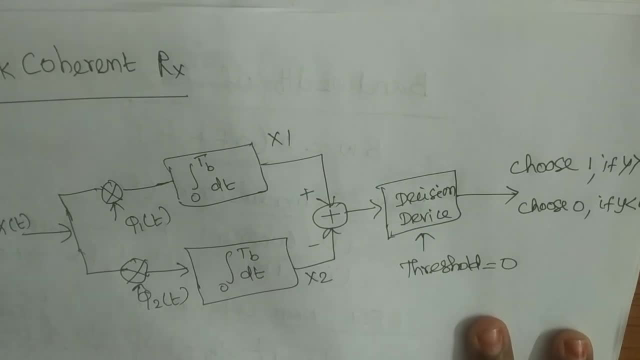 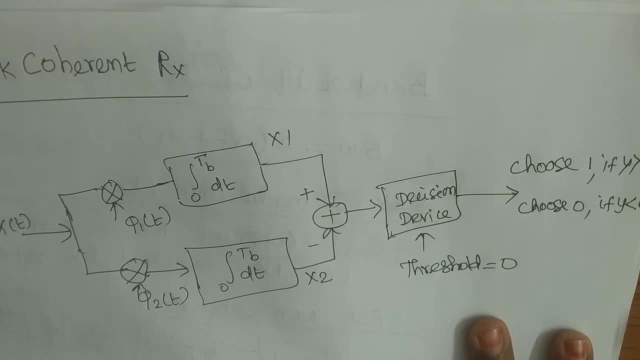 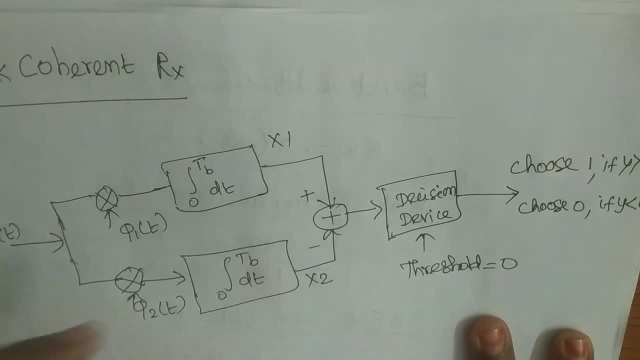 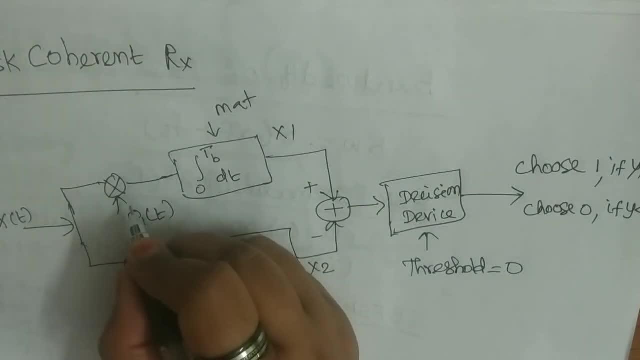 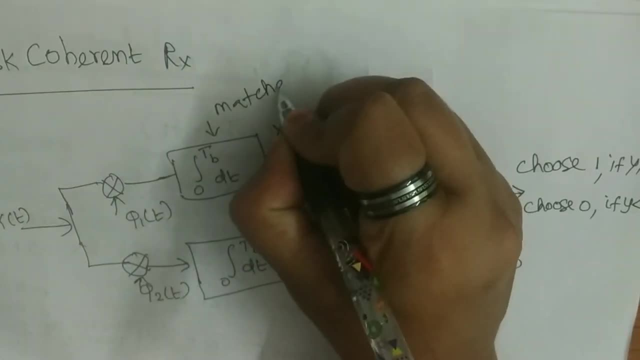 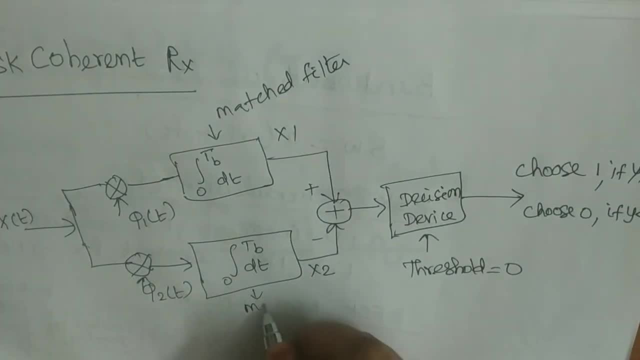 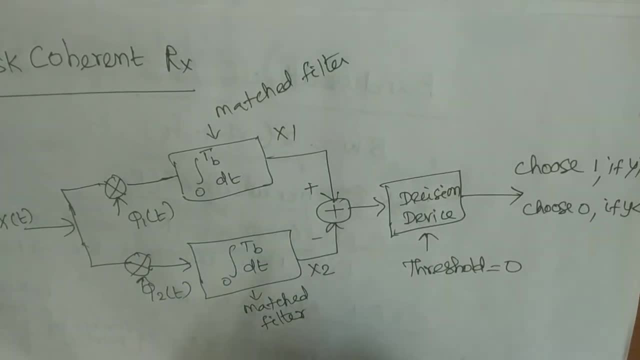 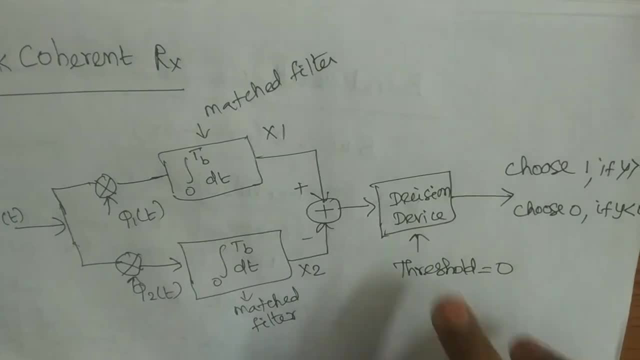 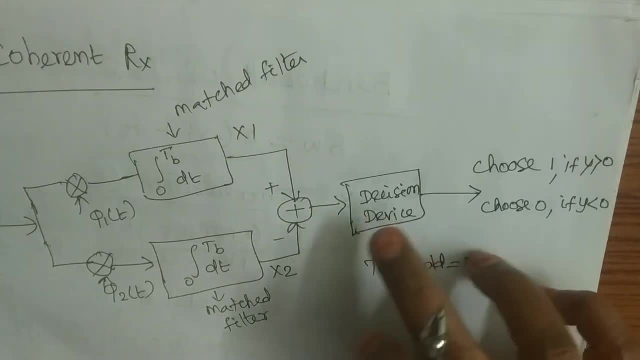 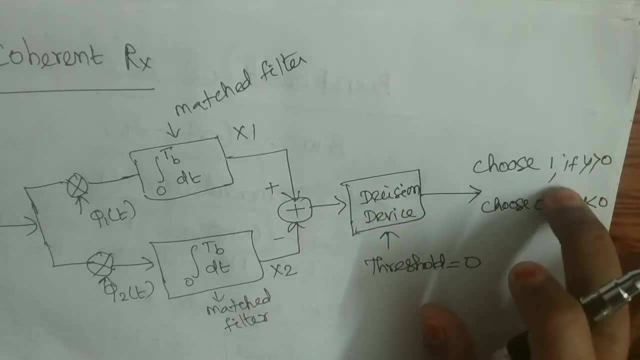 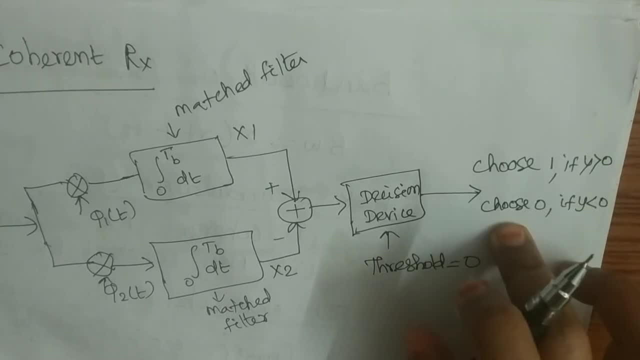 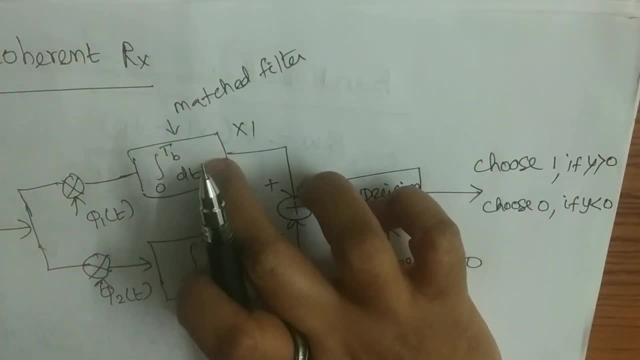 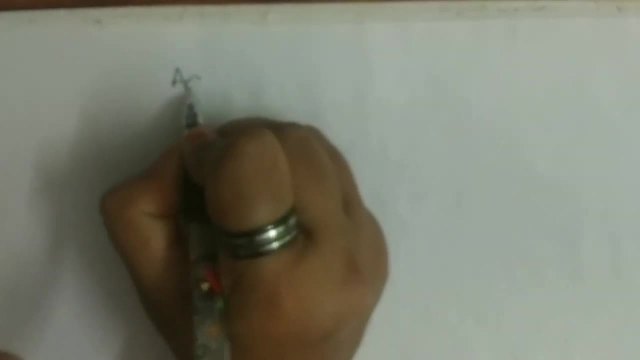 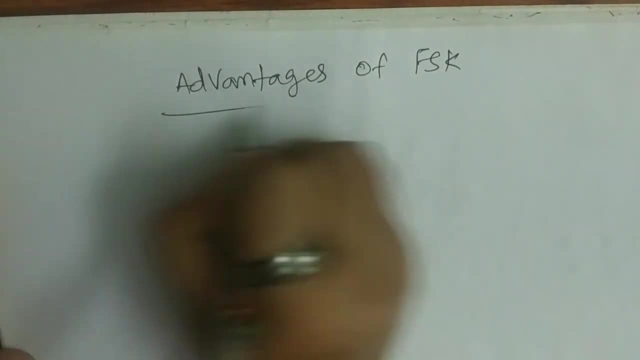 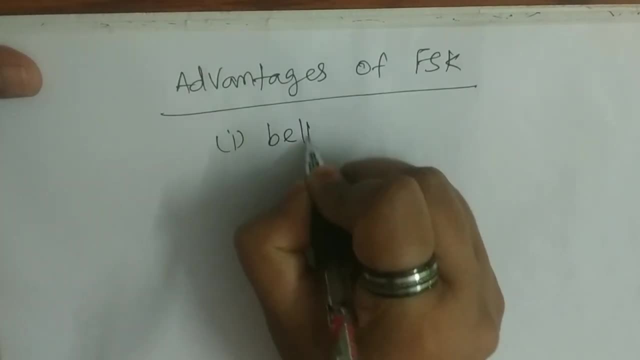 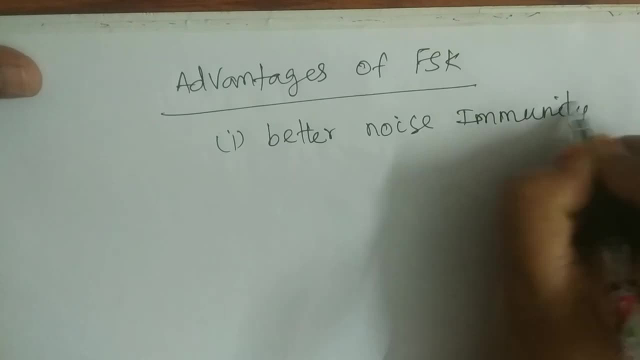 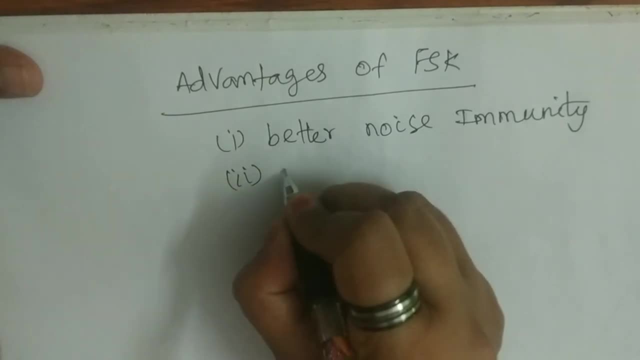 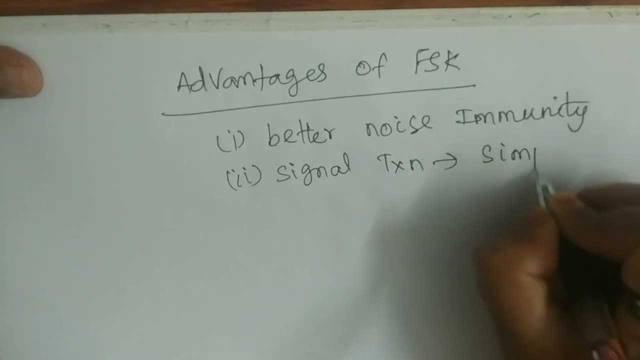 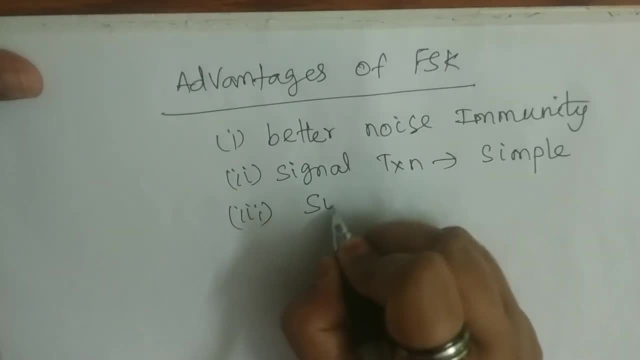 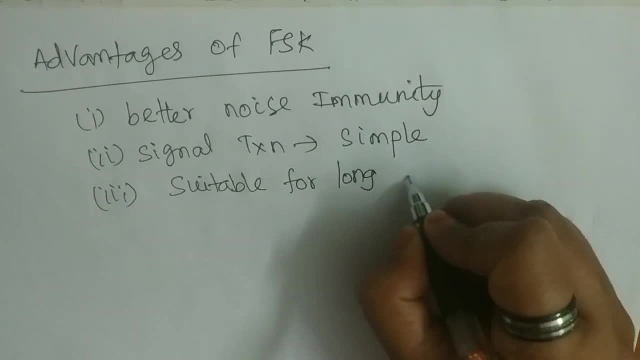 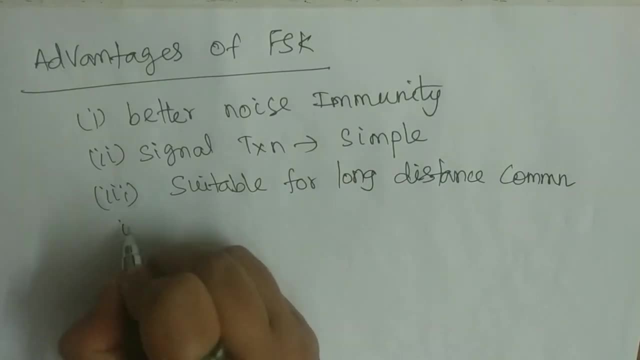 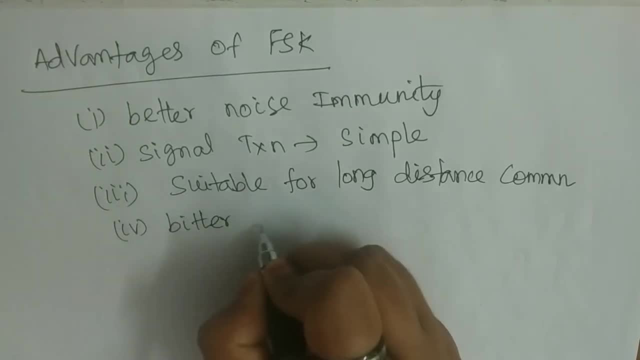 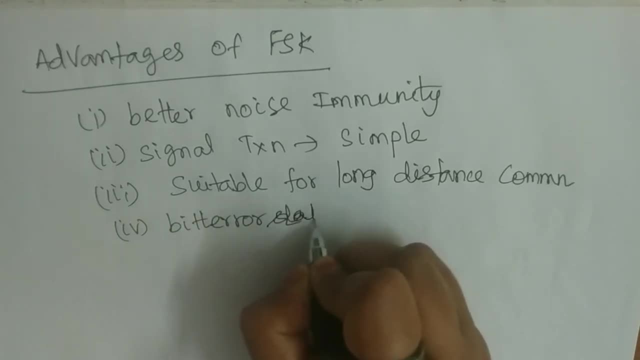 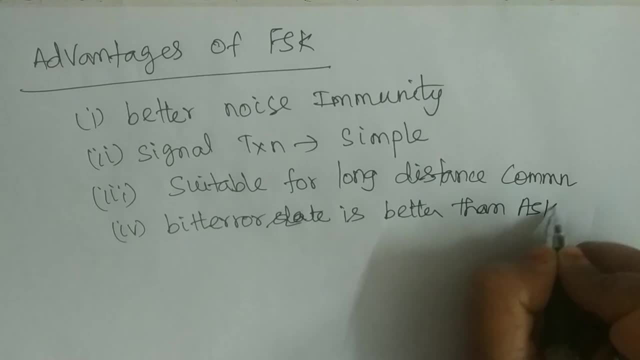 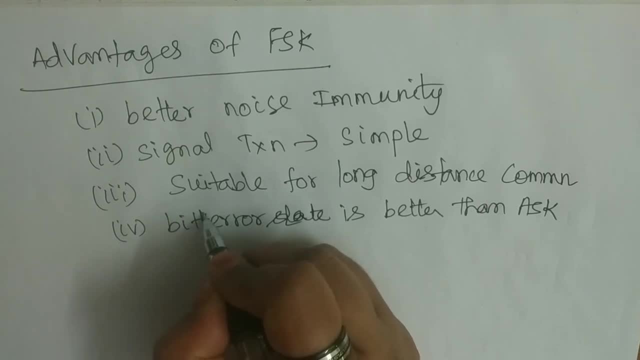 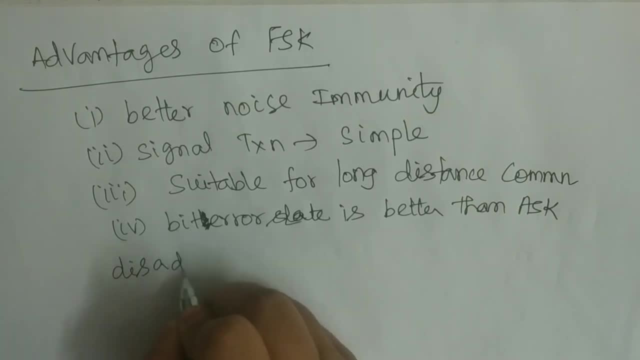 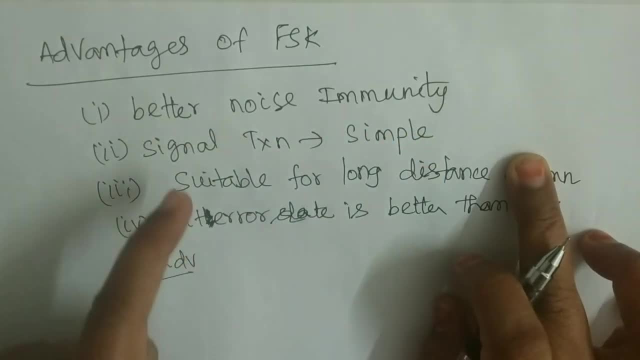 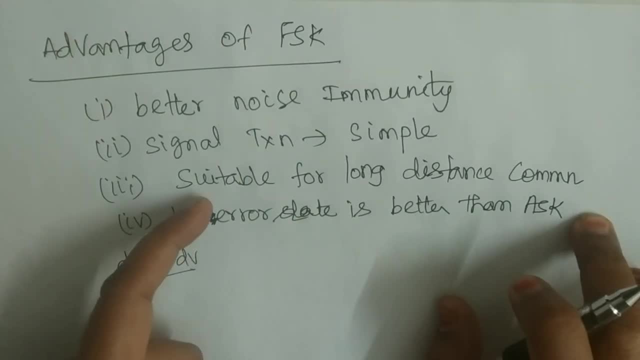 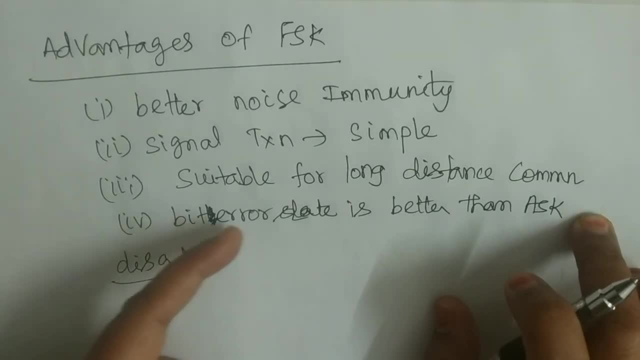 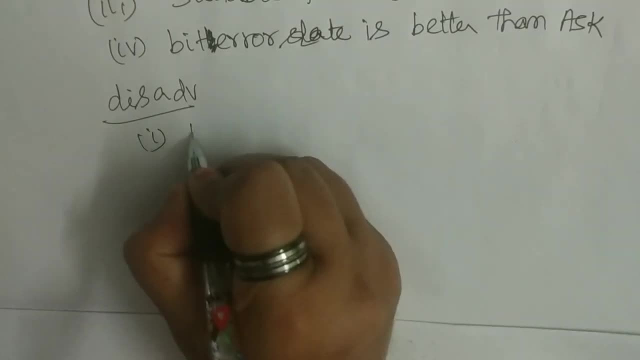 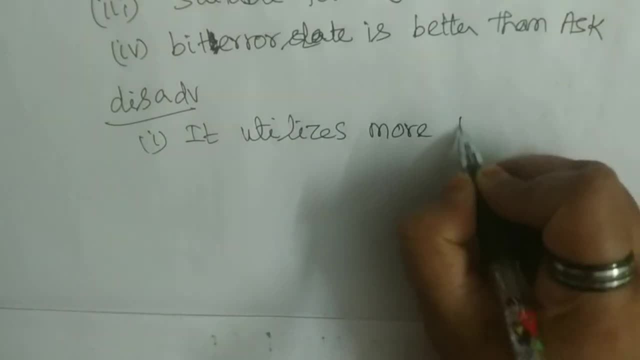 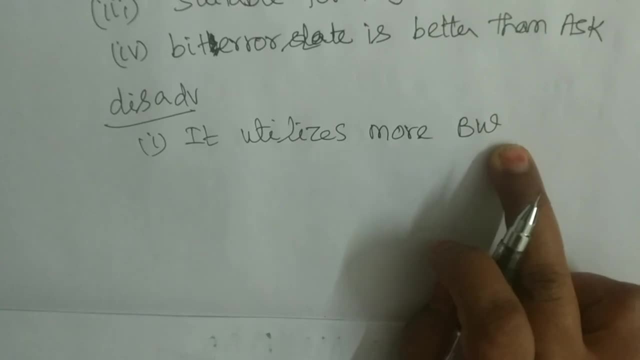 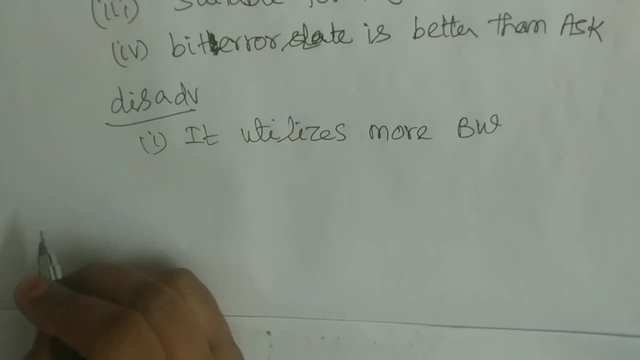 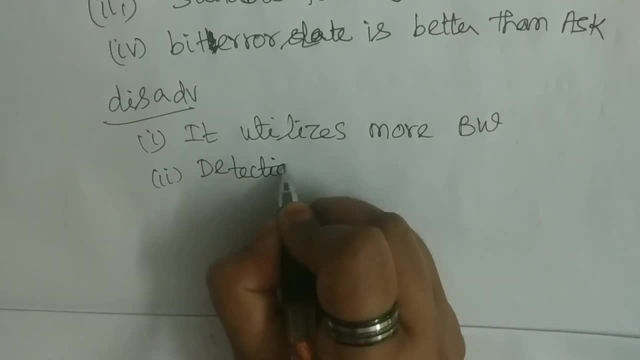 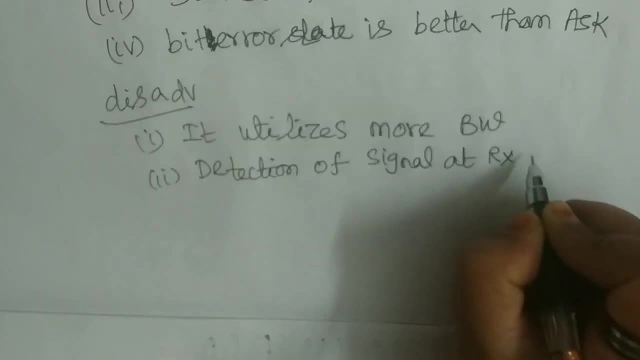 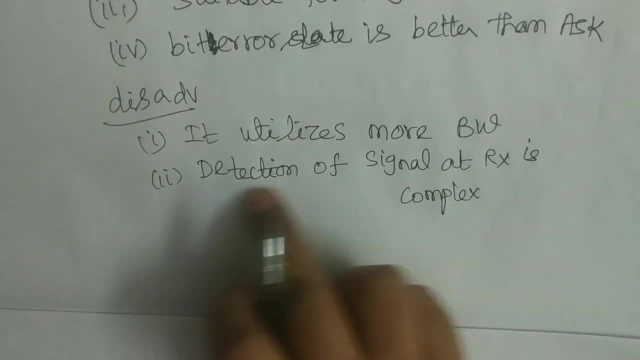 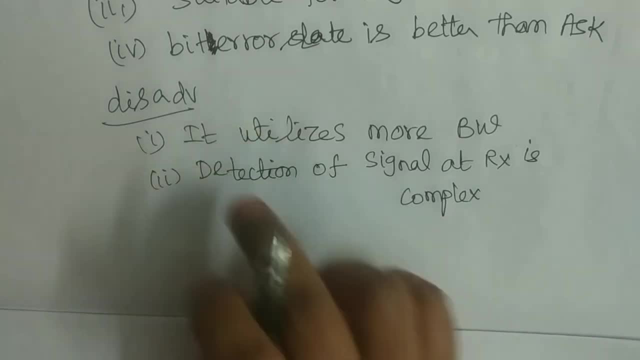 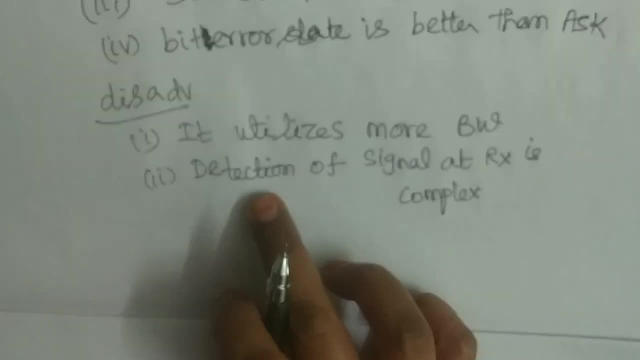 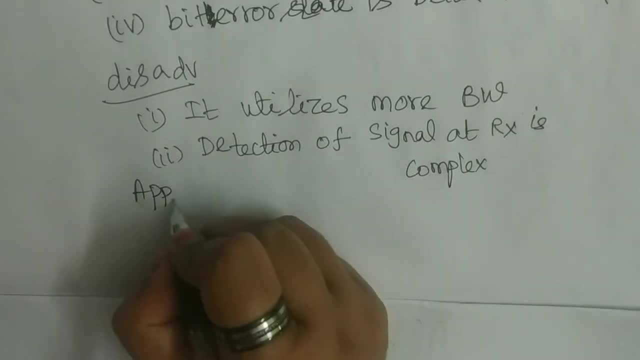 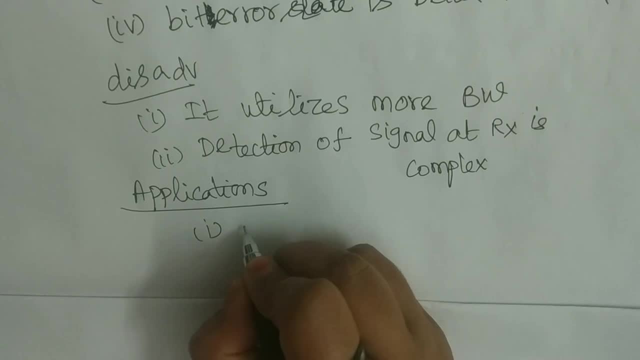 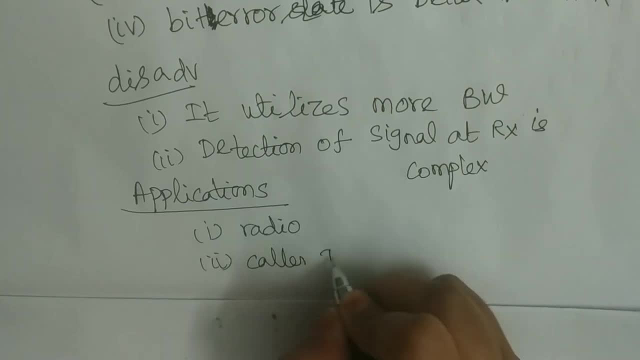 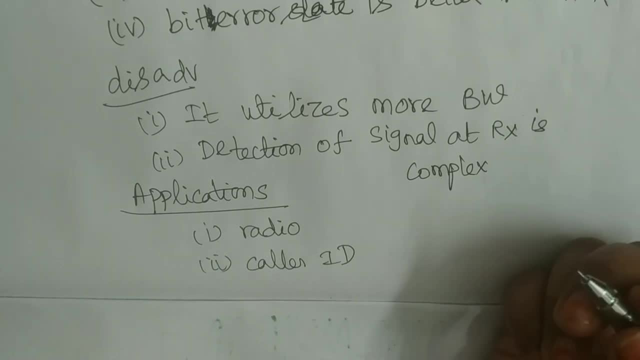 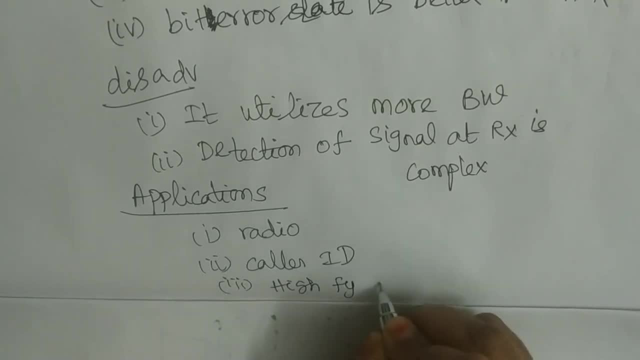 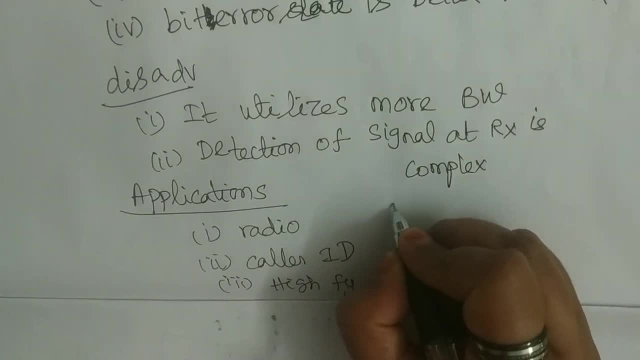 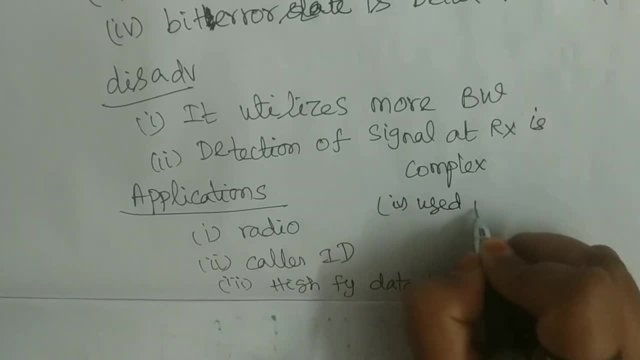